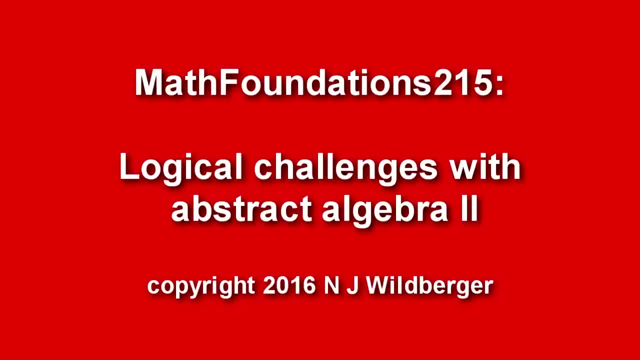 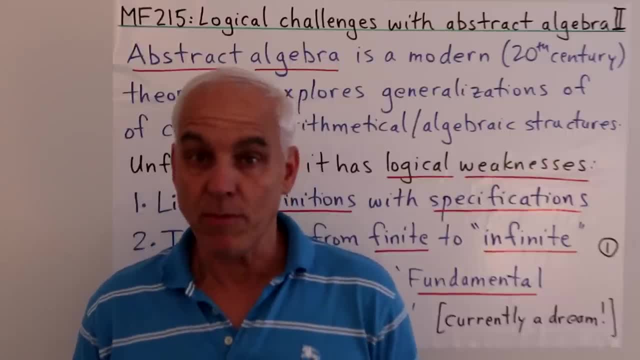 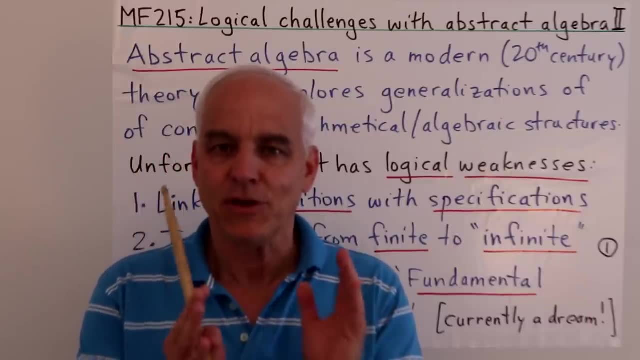 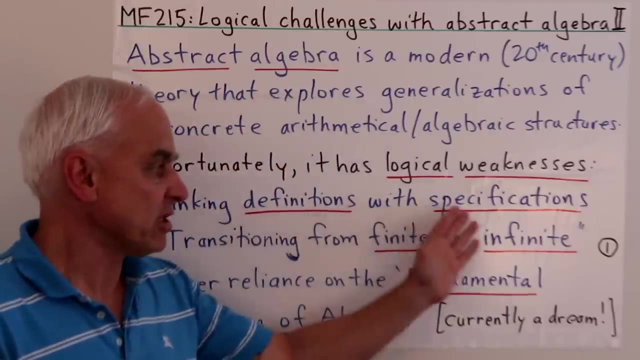 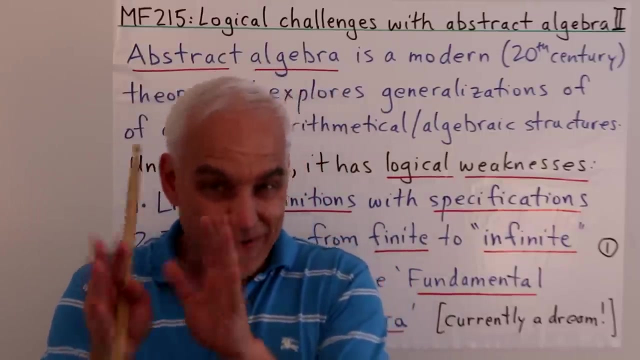 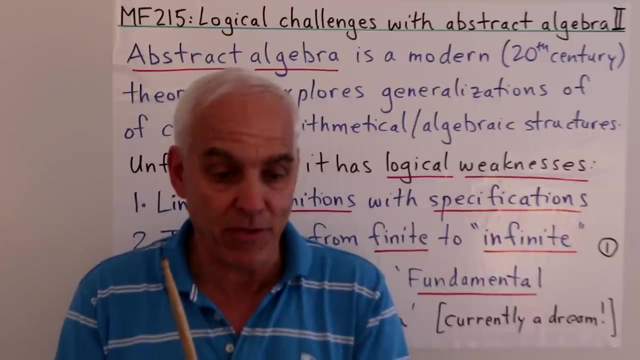 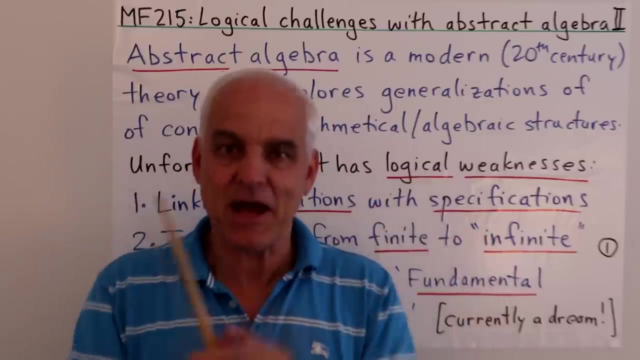 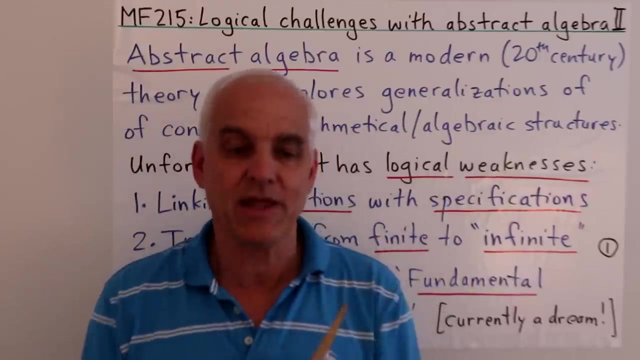 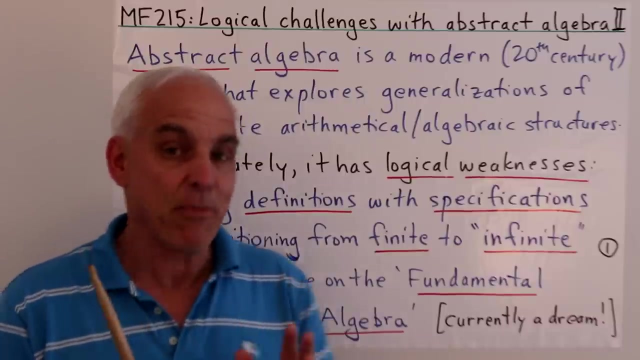 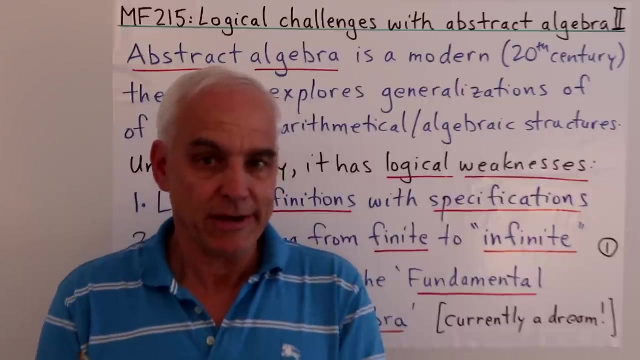 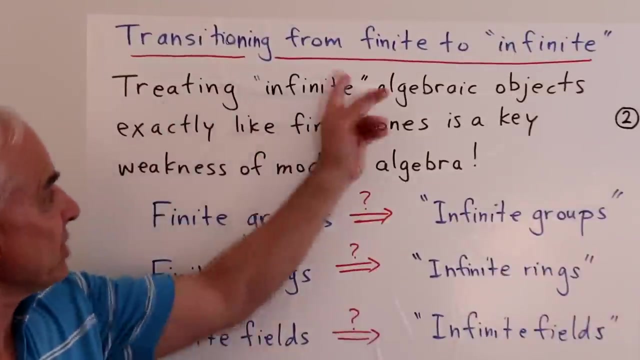 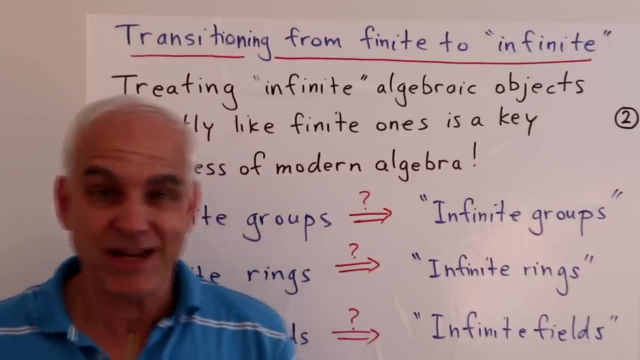 Good day, I'm Norman Wahlberger. Today we're going to carry on with our laying out of some fundamental logical weaknesses with modern abstract algebra. Last time we talked about the issues with definitions and specifications. Today I want to concentrate on the very big jump in trying to go from talking about finite objects to infinite objects. So currently when we say infinite objects we have quotation marks around them. That's not necessary in all cases. Perhaps we can create infinite kinds of objects but we have to do so carefully and ultimately in a finite way. So we may have to have a workaround. Okay and that's going to be part of the story here. So today I want to talk about a particular example that illustrates both some interesting aspects of finite group theory and then moving on to infinite group theory. We're going to employ a little bit about matrices as well which should be interesting. So this issue of transitioning from finite to infinite. So with current modern algebra we are often treating infinite algebraic objects with the same framework as finite ones. 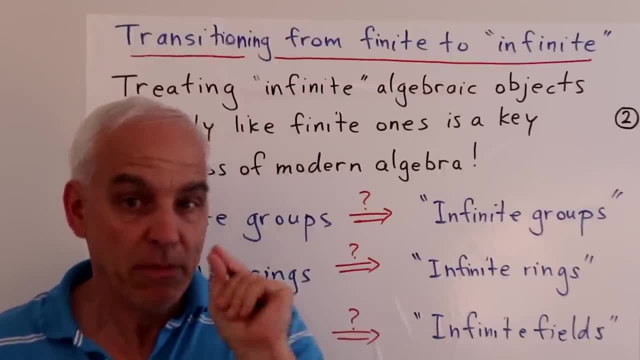 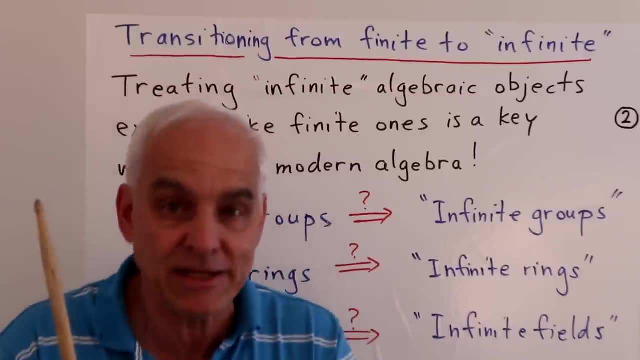 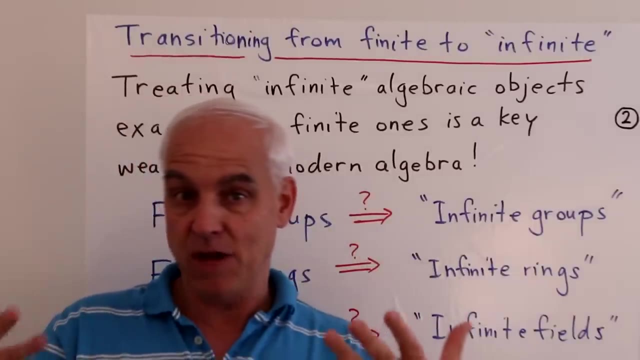 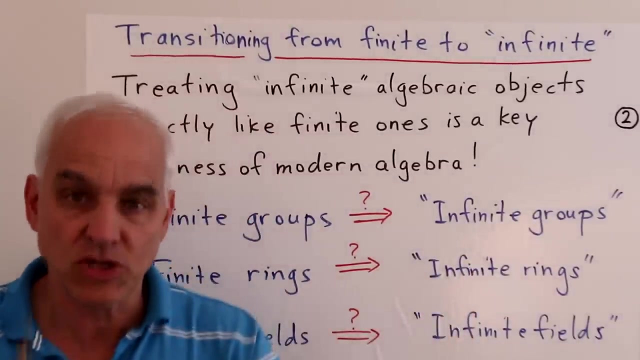 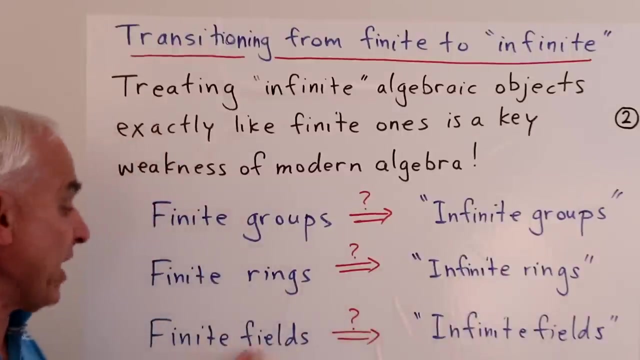 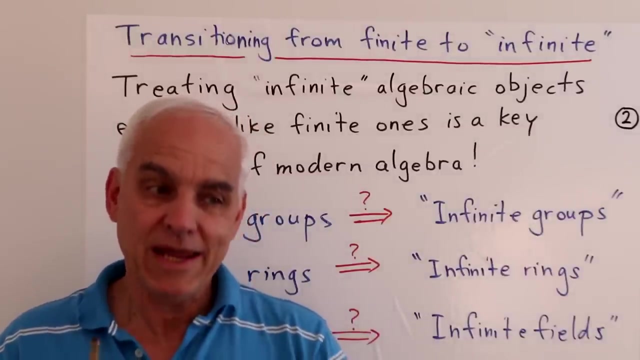 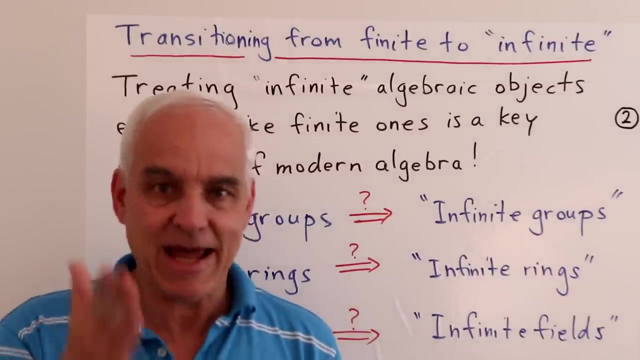 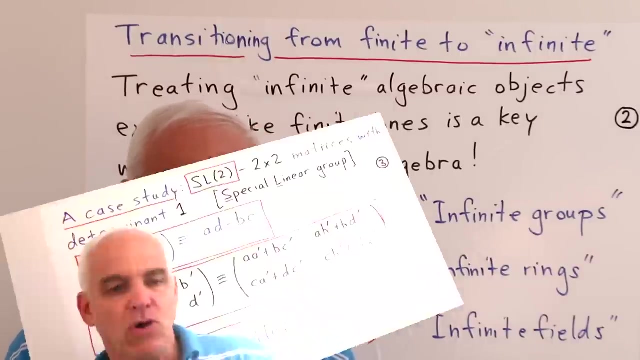 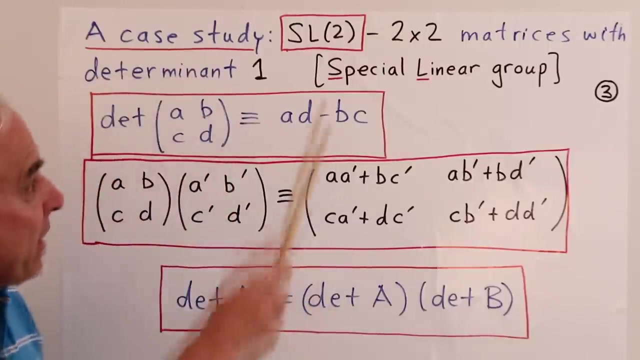 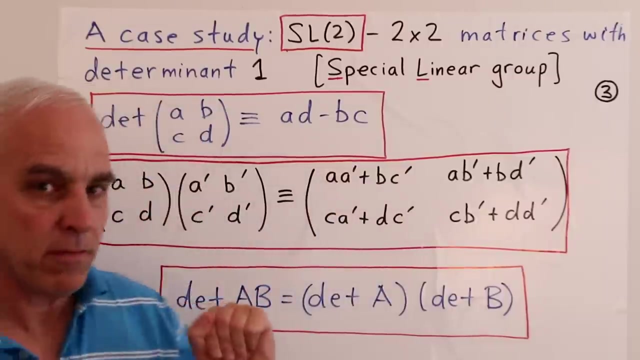 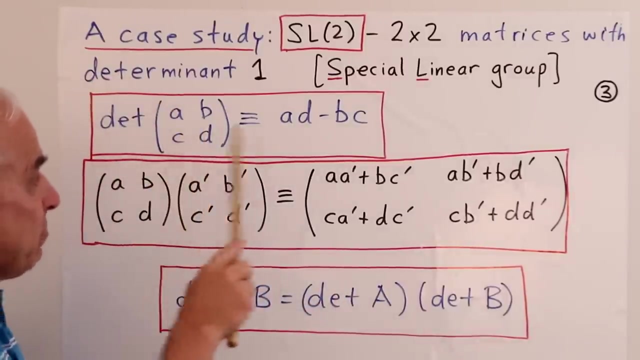 This is almost invariably a result of sloppy thinking. So the strategy is that if our basic definitions are fuzzy enough and imprecise enough then yes we can hope that we cast a big enough net so that both finite and infinite objects are embraced at the same time. But in fact going from finite groups to infinite groups is a huge step and requires really different separate thinking. Same thing going from finite rings to infinite rings or from finite fields to infinite fields, in fact pretty well everywhere, abstract algebraic object has the same problem okay we need different kinds of thinking we need often a more general kind of framework that gets at infinite procedures in a finite way so we have to think more carefully and often we have to be a little bit clever so I want to illustrate the issues at hand by looking at group theory and a particular interesting example that of SL2 so that's the context of 2x2 matrices with determinant one the SL stands for special linear so this is the special linear group okay so let me remind you of a few basic facts about 2x2 matrices first of all the matrix ABCD has determinant AD minus BC that's a number associated to a two by two matrix and 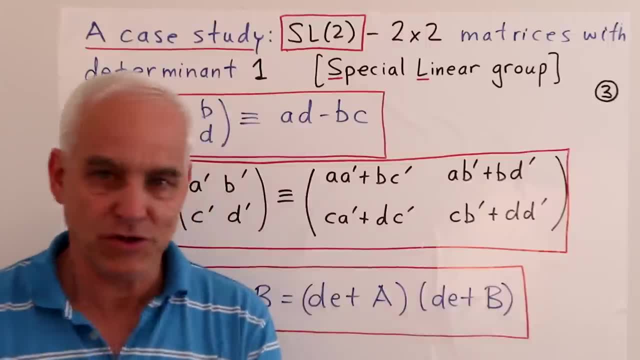 here is the familiar product of two matrices and here is the basic rule about 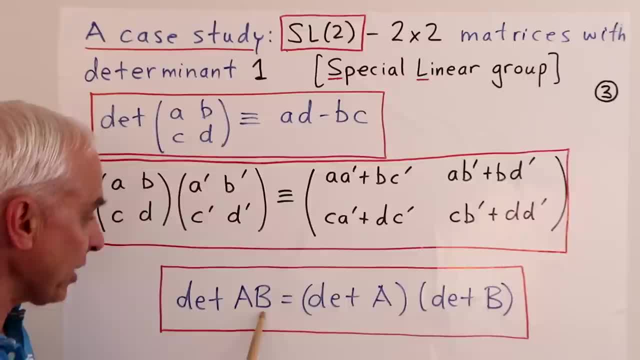 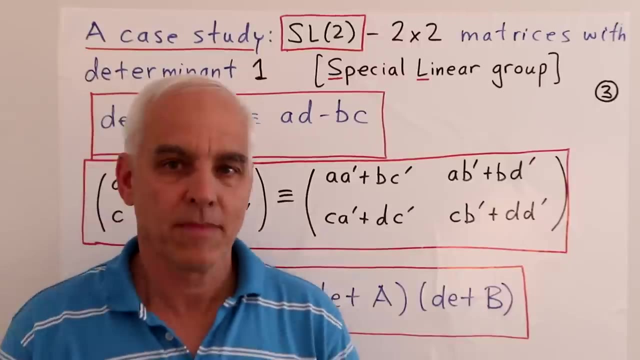 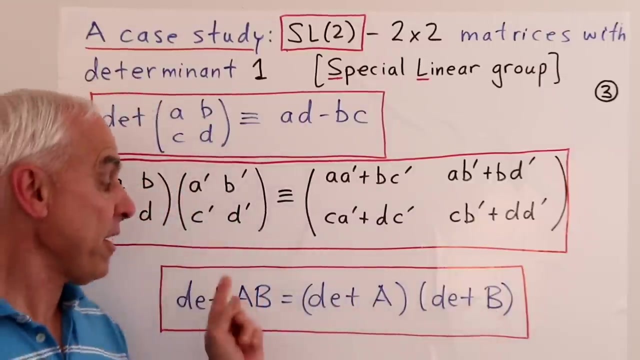 Ah It甦 determinants. That if you take the determinant of a product of two matrices, so A and B might be these two matrices, and then you take the determinant of this thing, it turns out to be the product of the determinant of A times the determinant of B. So this is the fundamental fact about determinants. In particular, if A and B both have determinant 1, then their product is also 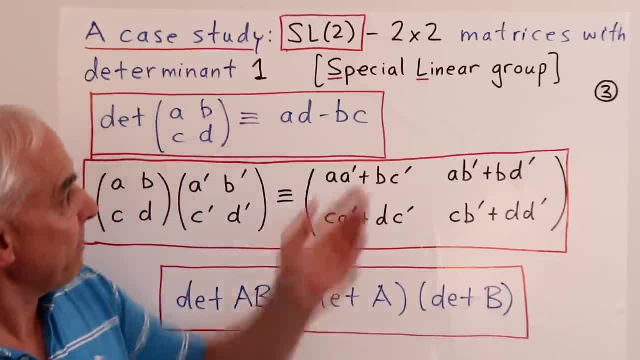 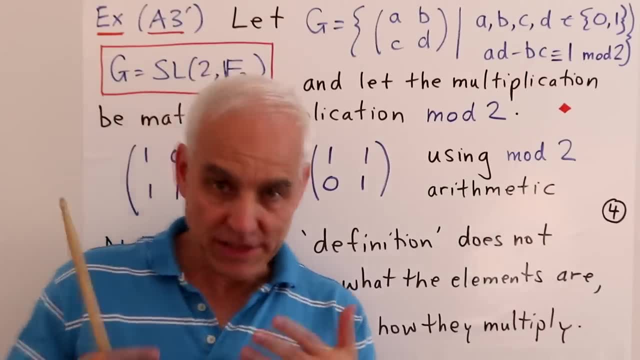 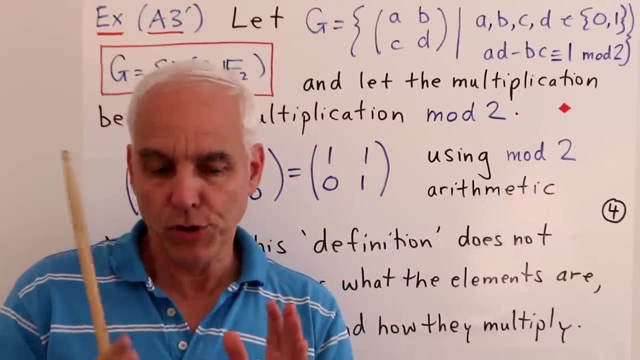 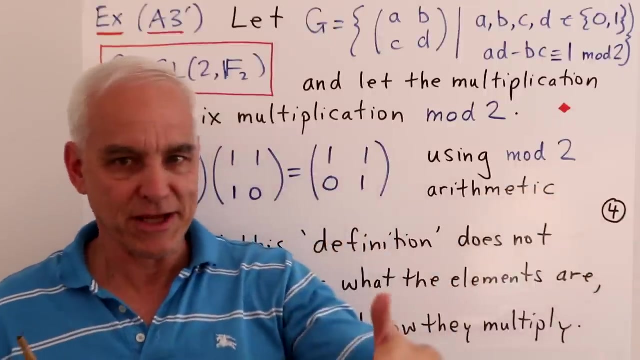 going to have determinant 1. That's the basic property that makes this kind of thing into actually a group. Okay, so now let's have a look at a rather specific case of two by two matrices with determinant 1, where we're looking at everything from the point of view of mod 2 arithmetic. In mod 2 arithmetic, it's a very simple kind of modular arithmetic. There are really only two values, 0 and 1. 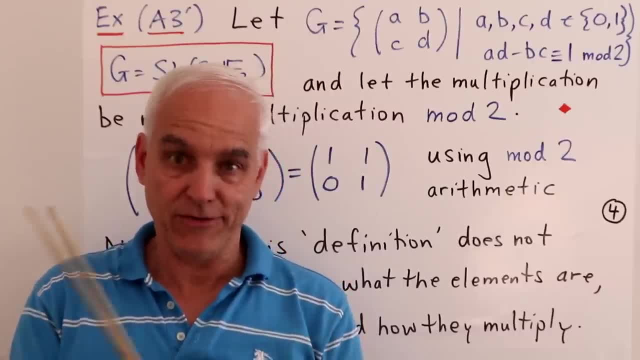 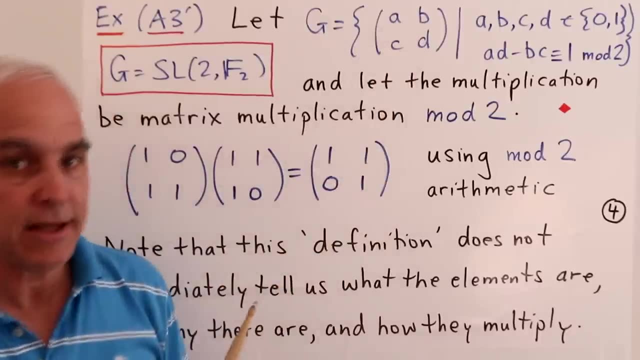 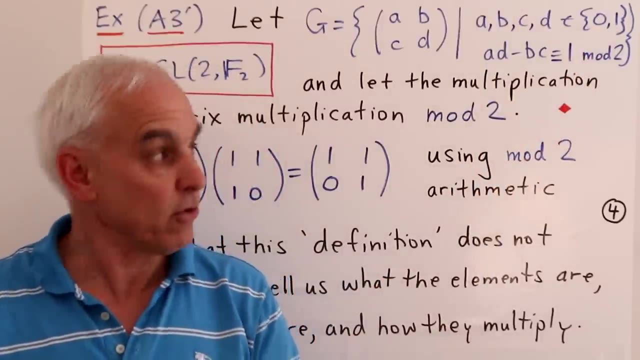 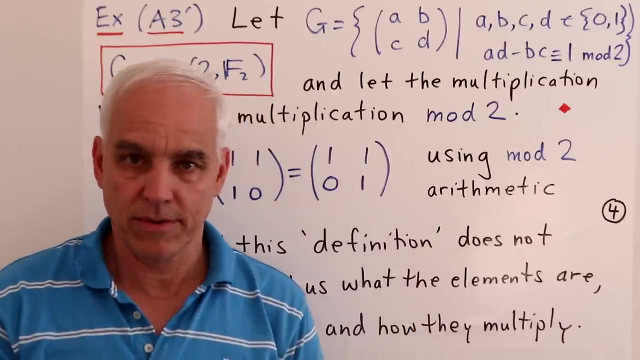 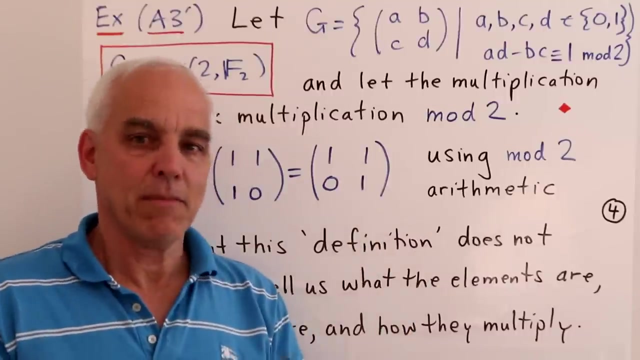 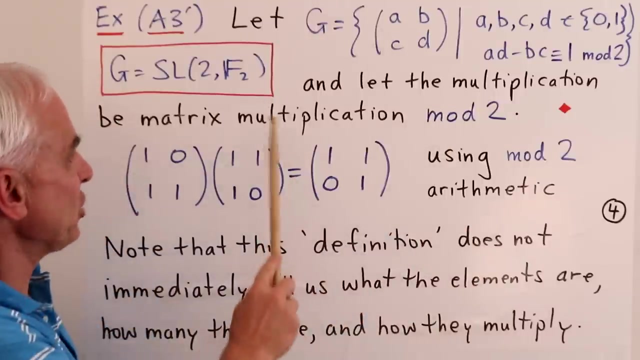 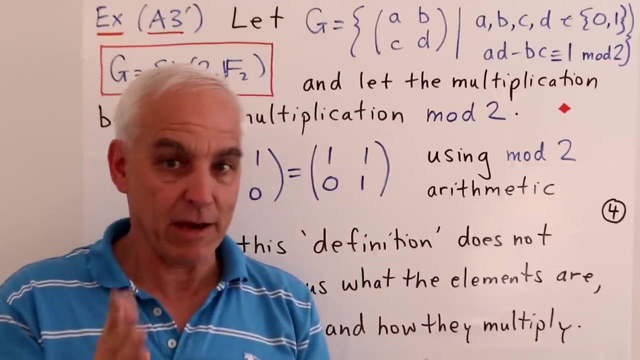 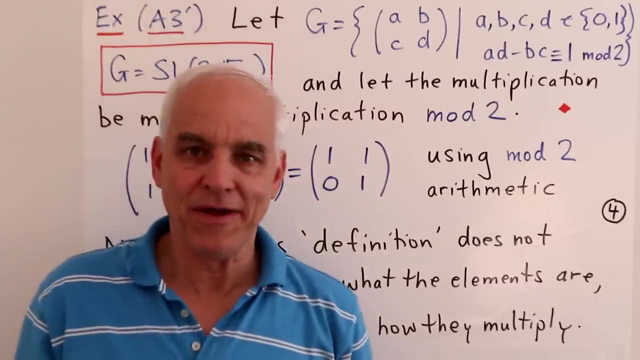 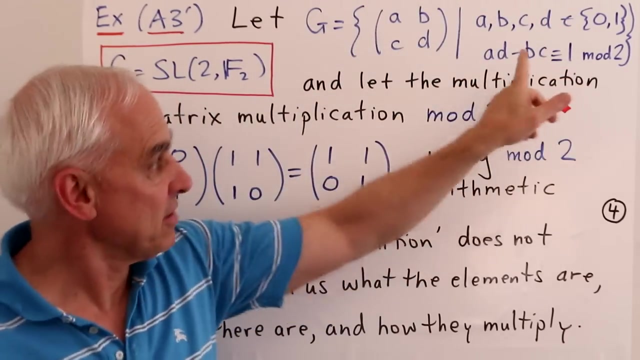 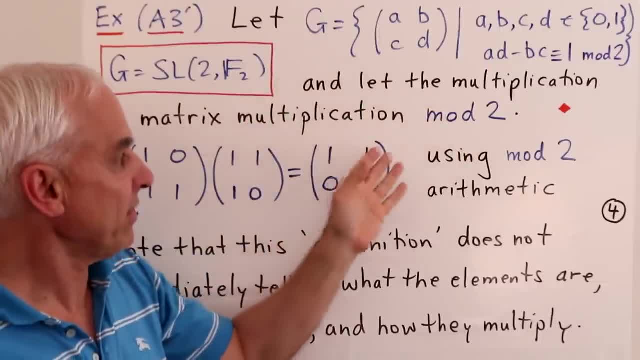 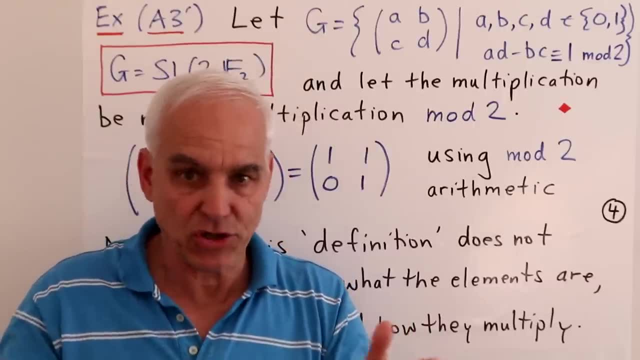 And also, well, we're basically sort of talking about what the multiplication is, instead of laying it out in the form of an array or a functional set. 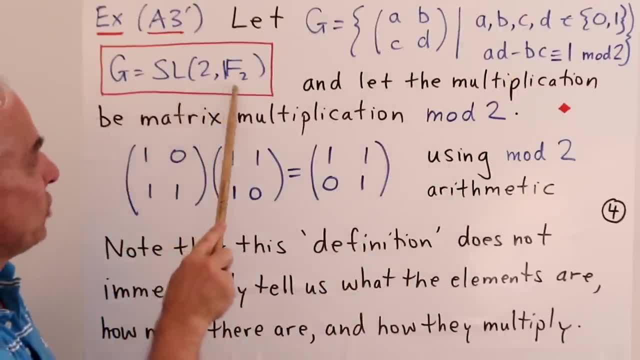 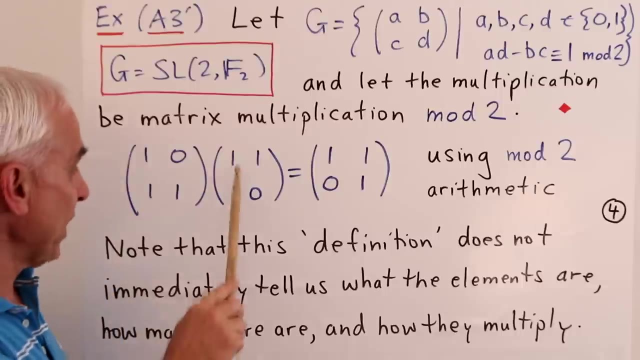 By the way, the name for this group is traditionally SL2F2, the F2 referring to the fact that we are basically working in a field with two elements. So for example, here are two matrices. This one has determinant 1 minus 0. That's 1. This one has determinant 0 minus 1. That's minus 1. 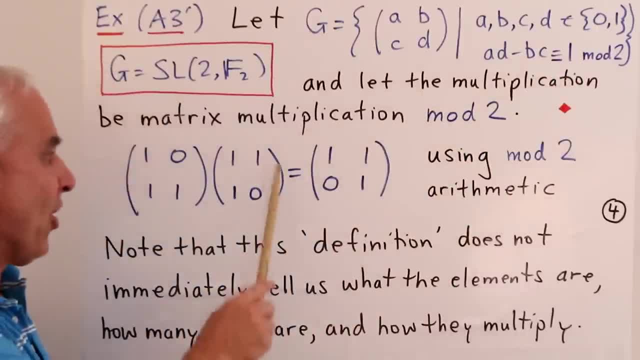 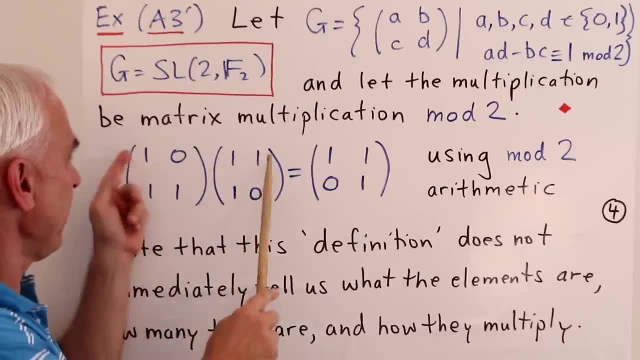 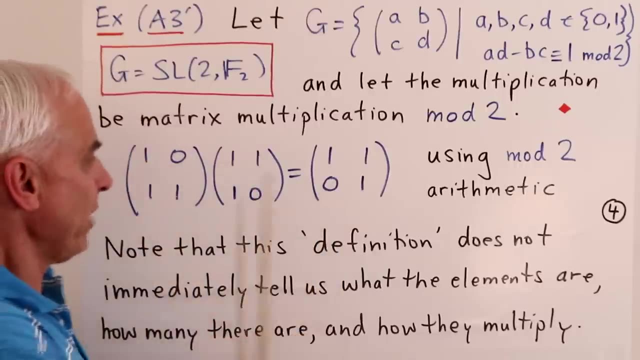 But minus 1 is the same as 1 mod 2. So this also is a matrix that belongs to this set. And the product is 1, 1, 1 plus 1 is 2, which is the same as 0. And 1 plus 0 is 1. And so that's also an entry of this set. 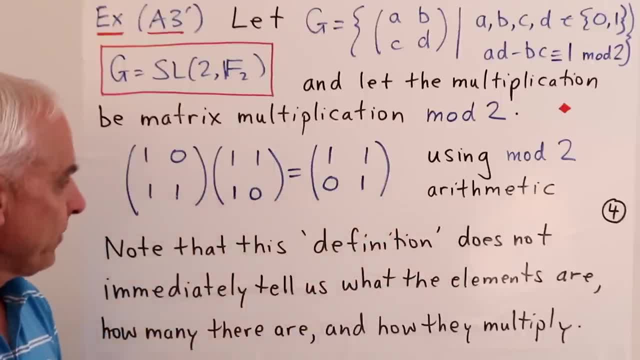 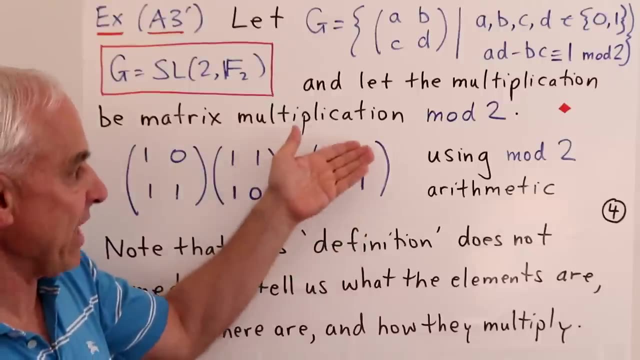 So we're using mod 2 arithmetic when we do the multiplication. So note that this definition, it's one of these A3 prime definitions. It's not very specific about what the set actually explicitly is. And it does leave us to understand what, or to compute what the multiplication is. 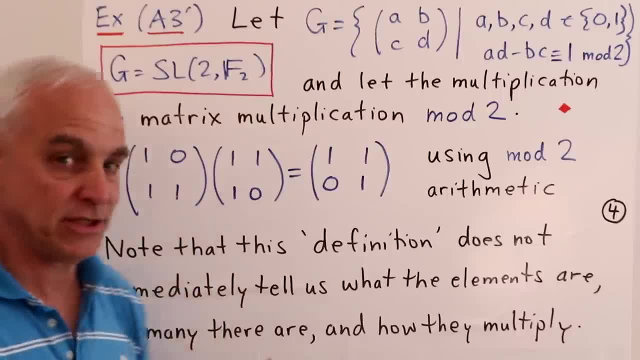 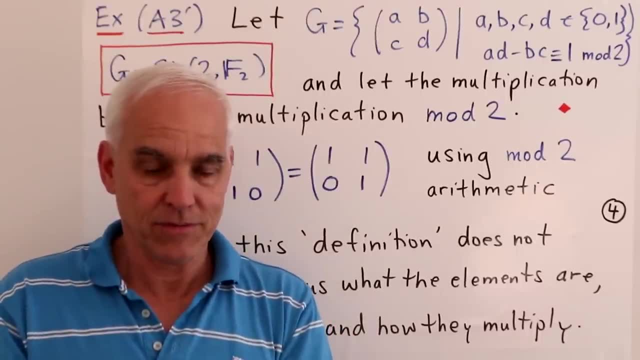 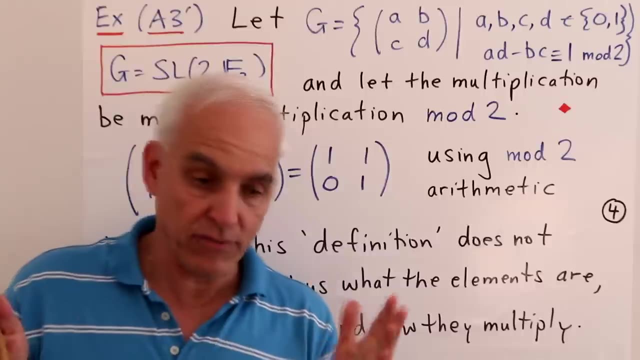 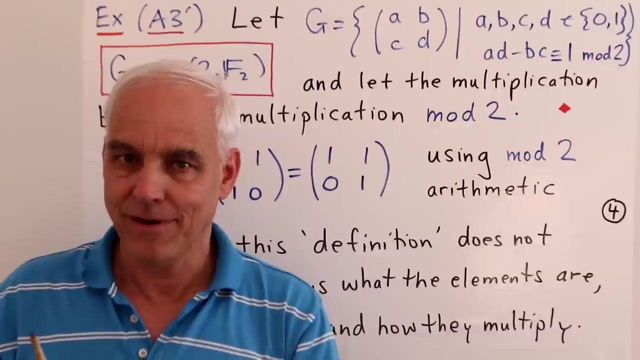 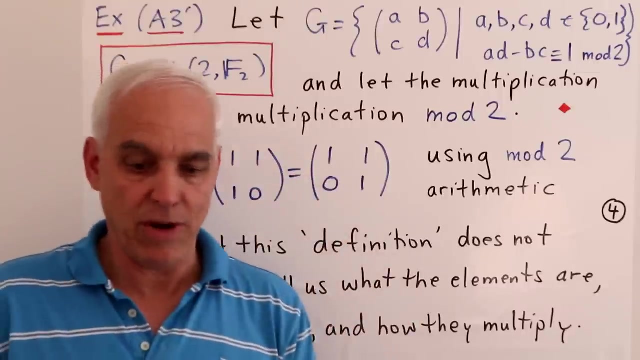 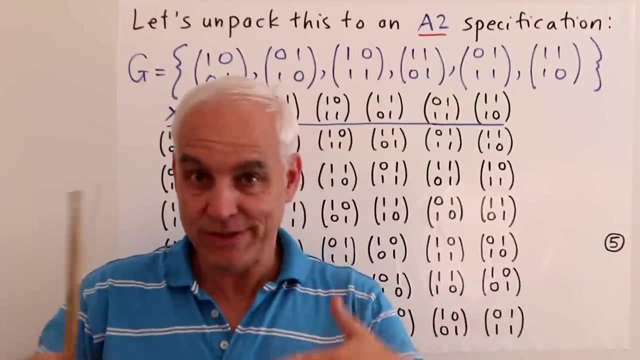 In other words, it's not telling us directly what the product of these two things is. It's giving us a recipe for us to be able to compute what the product is. So it's a different kind of structure than when you were given the multiplication table directly just as a table, and you're not required to understand anything more. You just look up stuff. Here we're asked to calculate stuff. So for a computer, this requires some more sophistication, because we have to know something about matrix multiplication in order to understand what this group is. So I want you to appreciate that different definitions really do lead to different kinds of things. Different kinds of group theory. 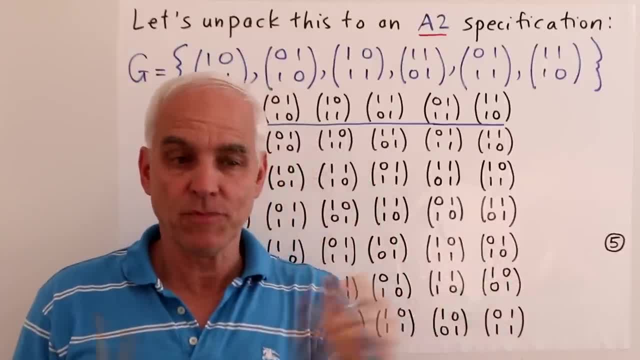 So let's unpack the previous A3 prime kind of definition to a more explicit A2 kind of specification. 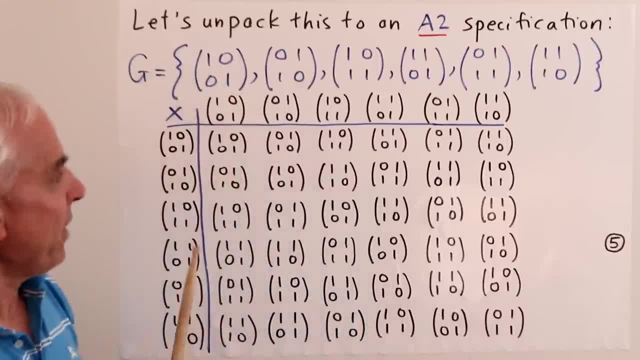 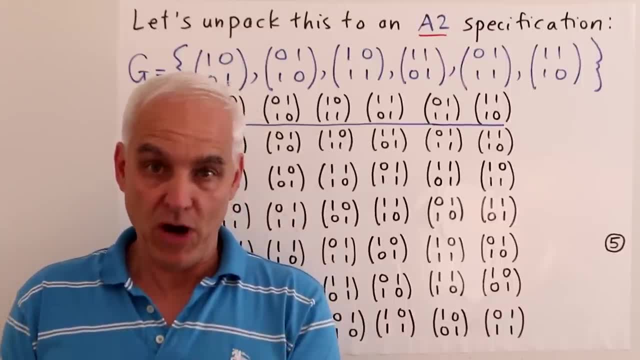 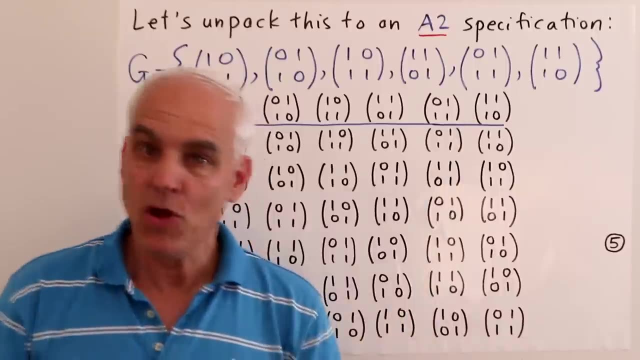 This is using the language of our previous video. So then what we need to do is we need to determine explicitly, first of all, what actually the elements of this group are. And here I've actually listed the elements of the group. It turns out that there's exactly six matrices. Made up of zero. 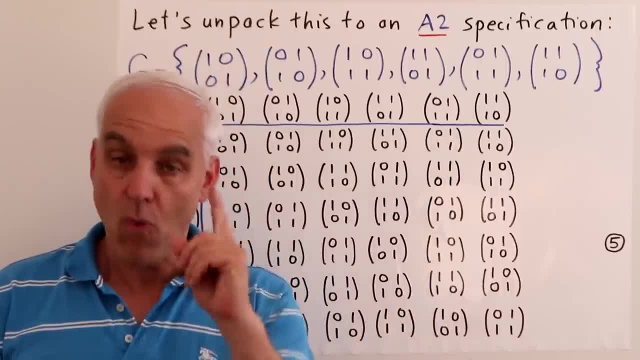 Zeros and ones that have determinant one. At least when you're working mod two. 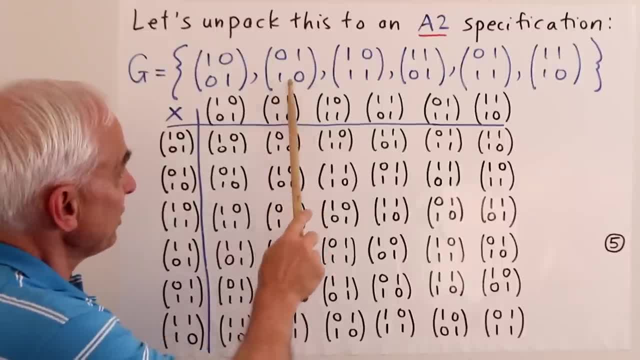 Here they are. There's the identity matrix. And then there's this one, which is a little bit like the identity, but sort of off diagonal. 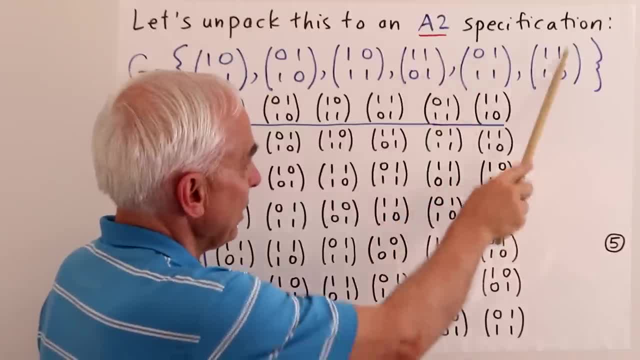 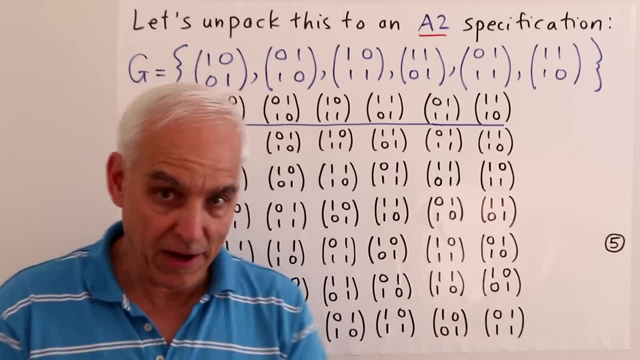 And then these other ones have a single zero in each of the four places and otherwise ones. And then here is a multiplication table, an explicit array that lists these elements in exactly that order. Both horizontally and vertically. And that tells you what the various products are. 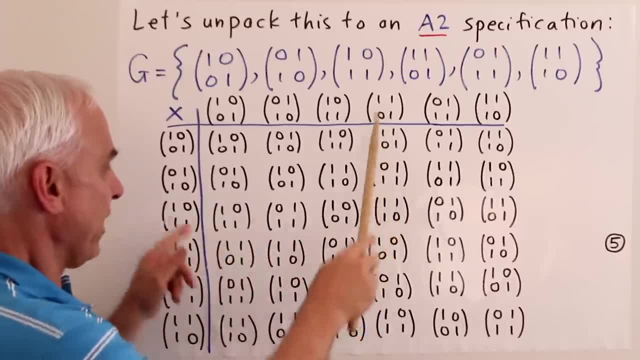 So the product of this matrix times this one is this one. You can check that hopefully I've done all the multiplications correctly. 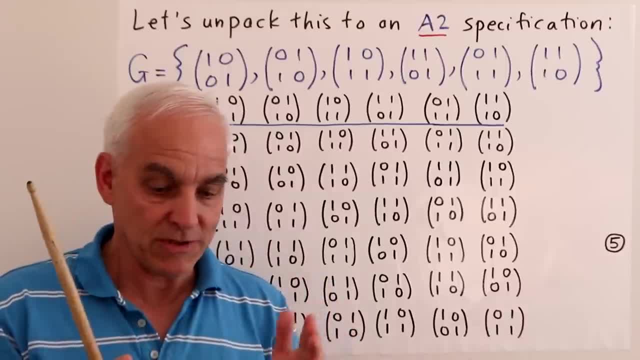 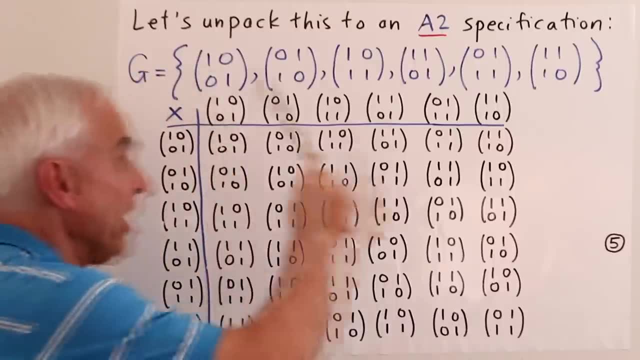 So if we were thinking about groups in terms of the A2 definition, then we would say, aha, here is the definition of this group G. Here is the set and here is the multiplication table. 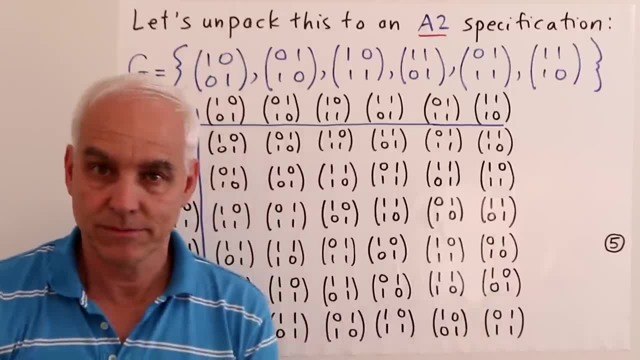 Even by this six by six array. It's different. 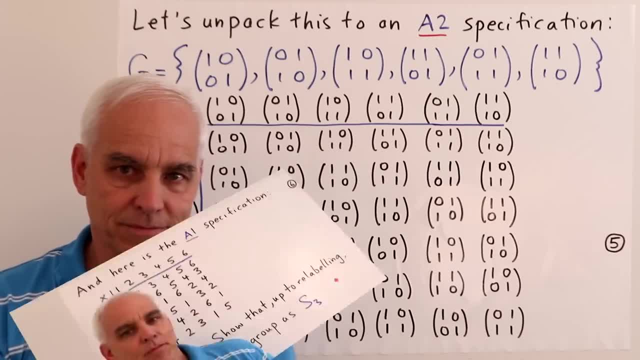 It's a different way of thinking about what a group is. 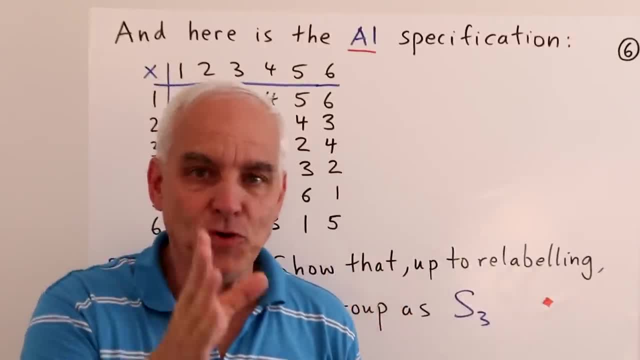 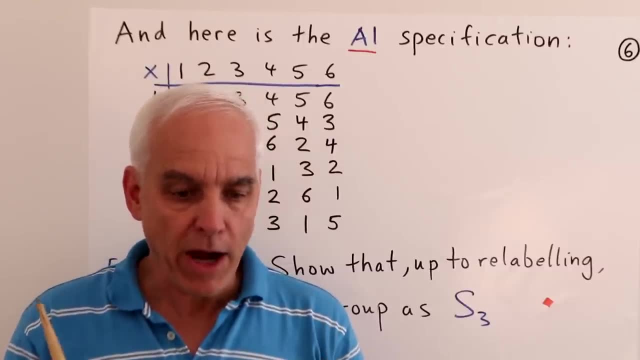 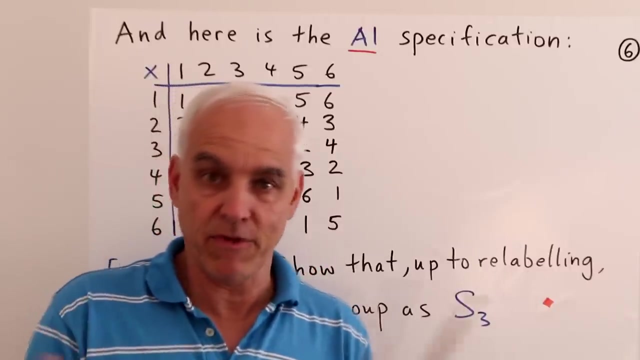 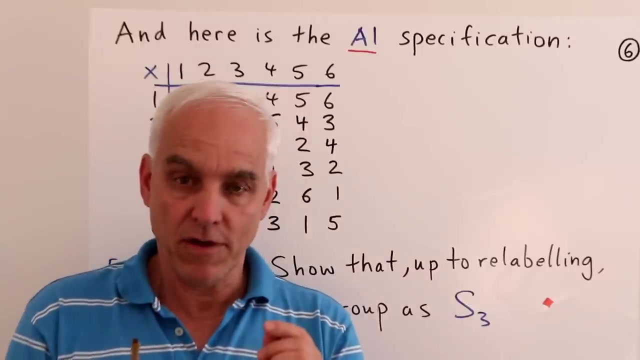 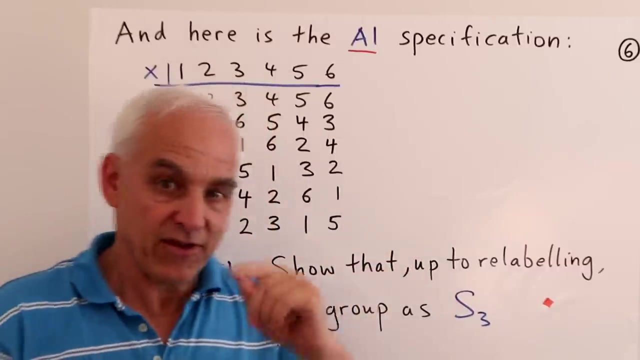 And now here is that same group, but viewed from the A1 definition. This was the most computer oriented definition, where we require that the elements be converted to just numbers one, two, three, up to K. Where? The number of elements in the group. And that we record just the array, the K by K array of multiplications in the language of one to K. So what I've done is I've just replaced the six matrices in the order that I gave you them in the previous slide with the numbers one through six. 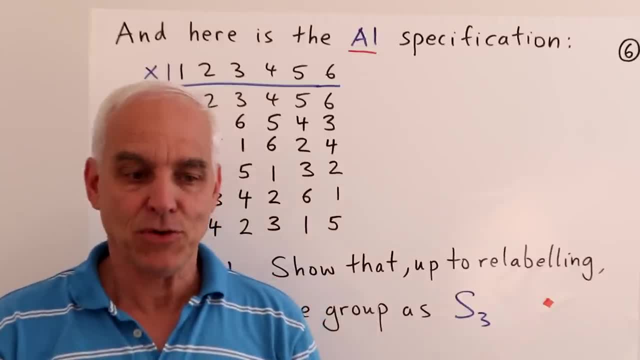 And I've just converted the table into a corresponding multiplication table. Now for the numbers one through six. Okay. 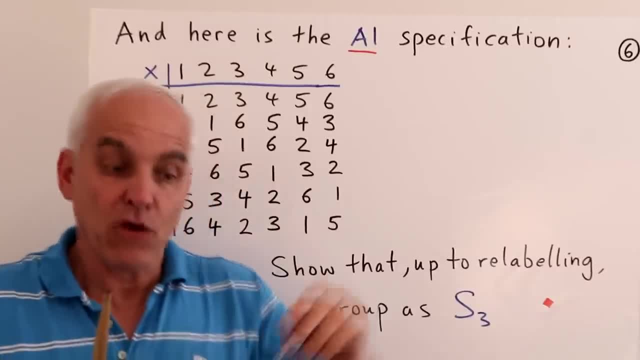 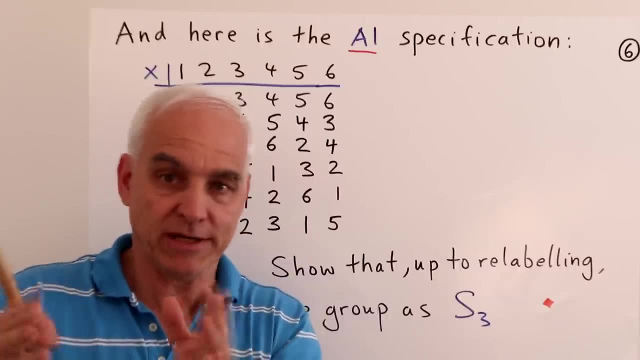 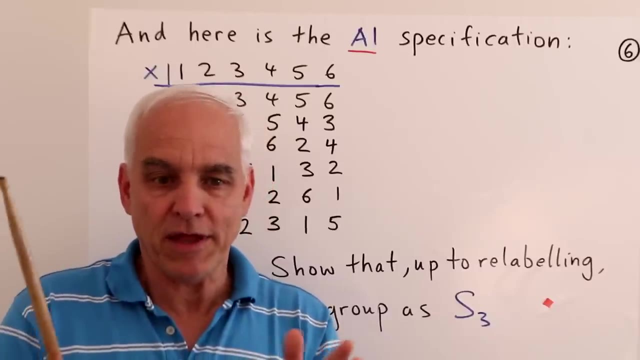 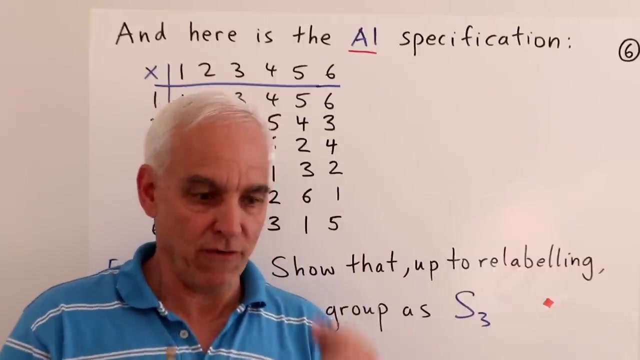 So notice that we've lost information because the original definition of the objects as two by two matrices with a certain determinant, et cetera, and the original matrix multiplication mod two formula for the multiplication. These are now lost. We no longer see them. We just see the bare bones algebraic structure of what multiplies to what to get what. So. Okay. 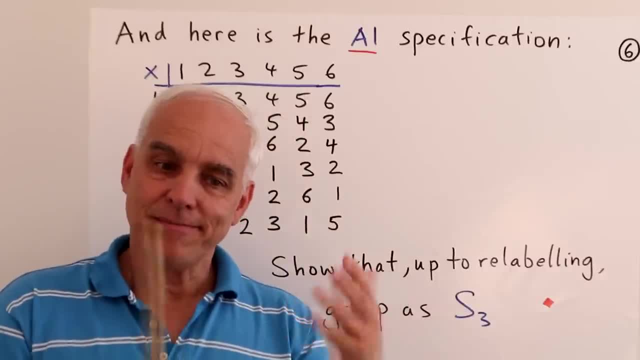 So this is a very efficient way of thinking, but it does really look at things from just a pure algebraic point of view. Okay. 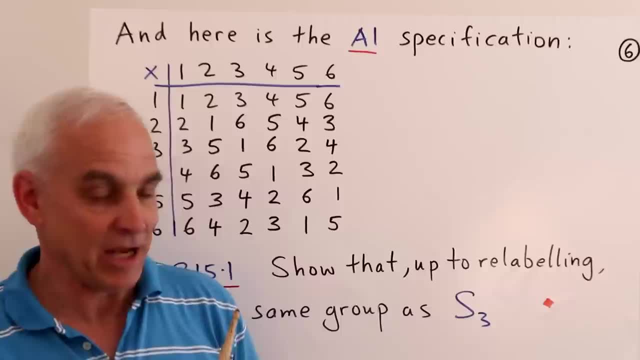 But this is a pleasant group with six elements. It's one that we should be familiar with. 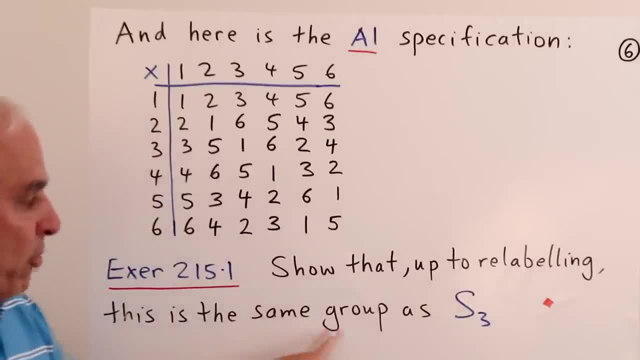 So as an exercise, show that up to relabeling, this is the same group as S3. It's the same as the symmetric group on three things, which we've seen before. Okay. 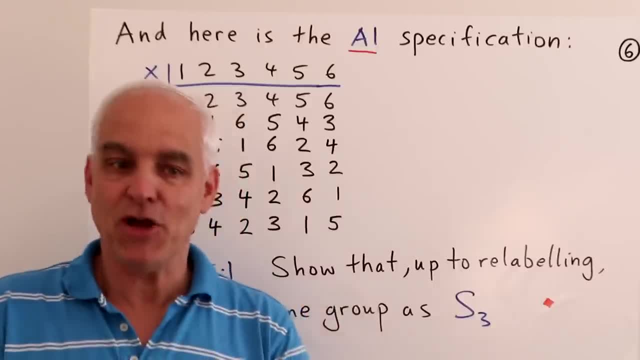 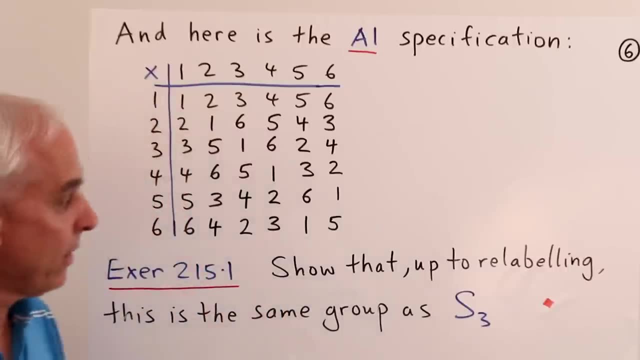 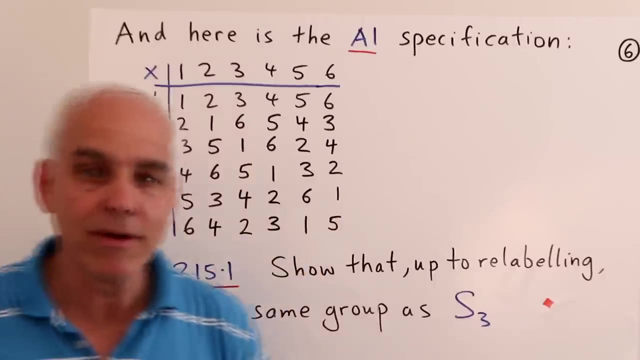 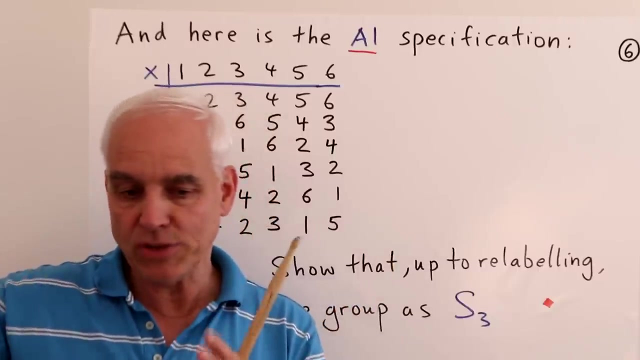 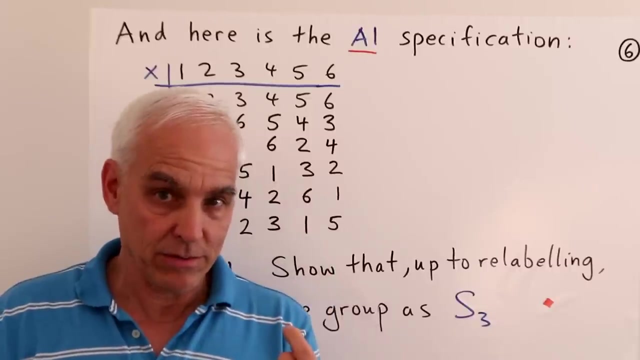 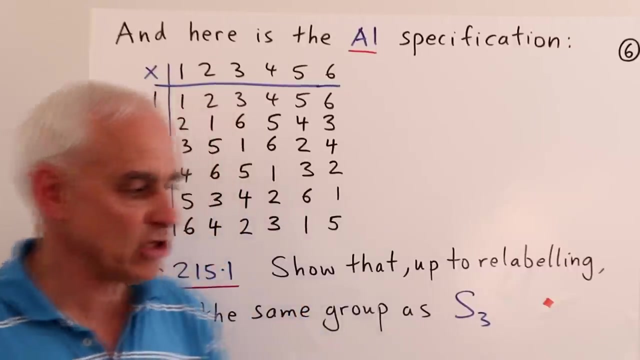 But it's now not in terms of permutations, not in terms of matrices, but just in terms of multiplications of the numbers one through six. I'm going to say up to relabeling, we should be aware that this particular multiplication table is what we've obtained by choosing a particular order of the elements, right? If we had chosen a different order of the six elements, then we would have gotten a different. We would have gotten a different multiplication table. So there's a little bit of subtlety here about how the ordering and choice of ordering determines the multiplication table. 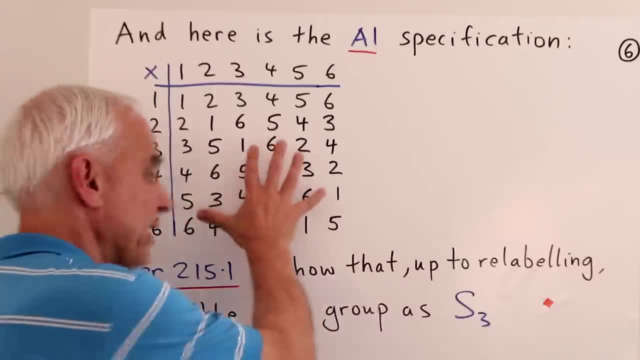 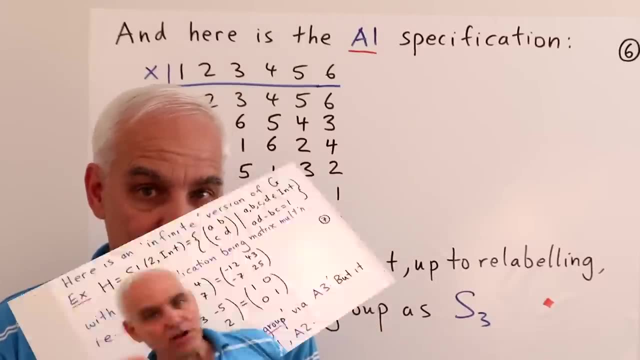 But from an A1 point of view, a group is just a multiplication table like this. Convince yourself this is really S3 in disguise. And so now let's make a jump from this finite group that we've been looking at to a sort of infinite version. 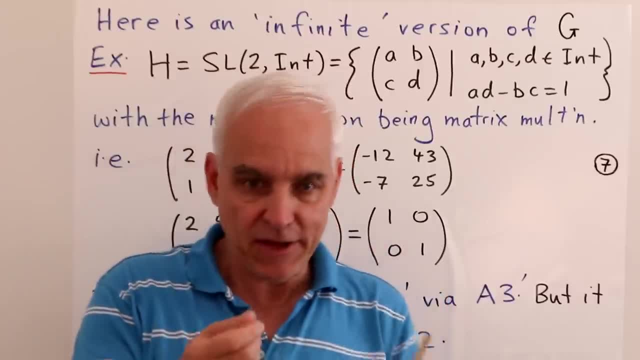 Okay. So we'll get an infinite version. Okay. We'll get an infinite version. Okay. So we'll get an infinite version. Okay. So we'll get an infinite version. Okay. 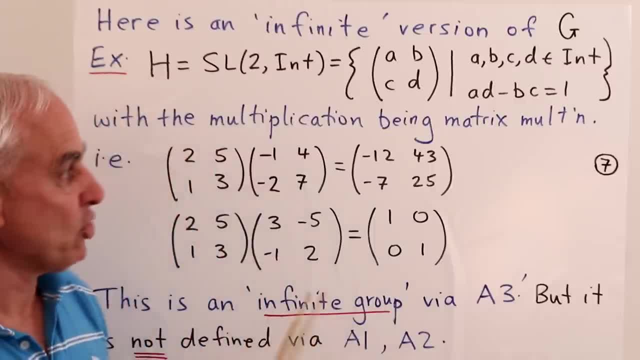 So this is the finite condition that the entries are just zeros and ones with a more general condition that will allow A, B, C, and D to be arbitrary integers. And we won't do mod 2 arithmetic, we'll do ordinary integer arithmetic. So the determinant has to be exactly 1. So this is now a new group H, let's say. 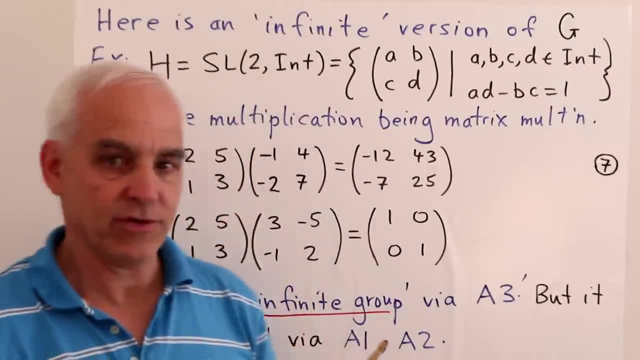 And its name might be SL2int because it's special linear group, determinant 1, with integer entries. 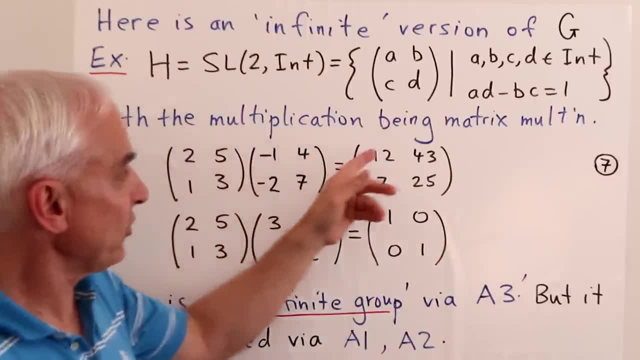 And we'll specify that the multiplication is just matrix multiplication. 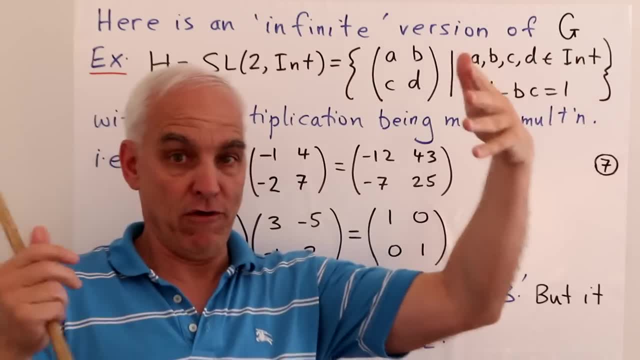 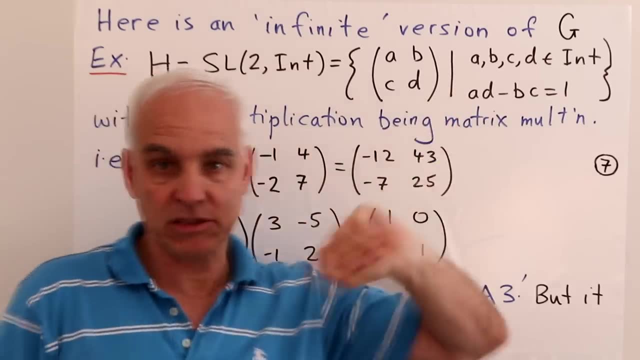 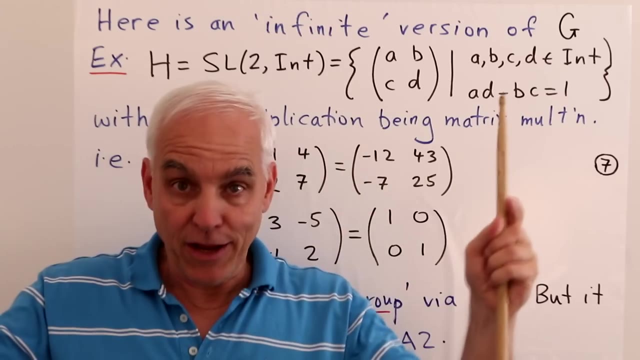 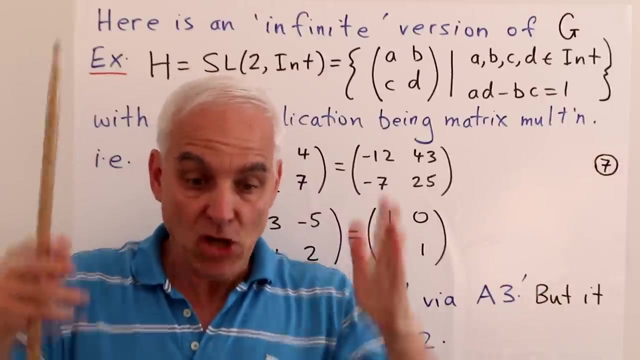 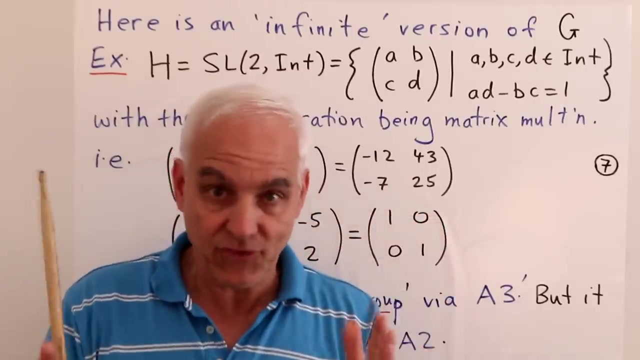 We are just giving a description of a set, a set in quotes, very big quotes, and a description of matrix multiplication as being the multiplication that's involved. We are definitely not exhibiting the set as a set, as a completed set, which all the elements are there for you. We are definitely not exhibiting the multiplication in terms of an array, where you can see the entire array in your database. 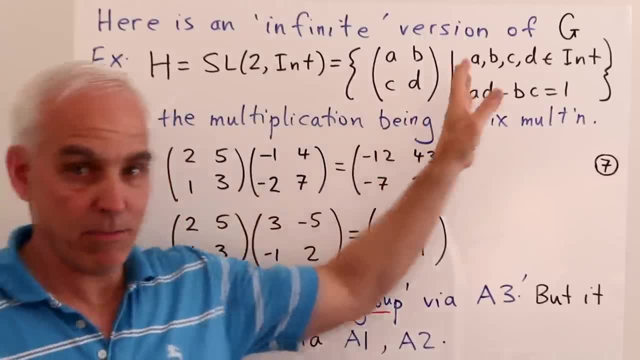 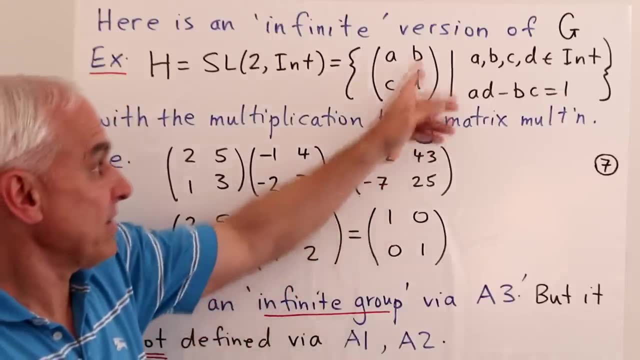 That's going to be impossible because there's going to be an unbounded number of such matrices. This is not a finite group. It's unbounded. And in particular, these... Integers can get very big. 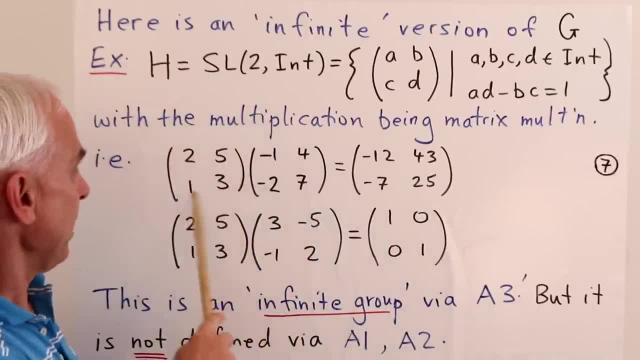 So, for example, here is a matrix with determinant 1, 6 minus 5. Here's another one with determinant 1. That's minus 7 plus 8. That's plus 1. So the product of these two matrices is that one there you can check. 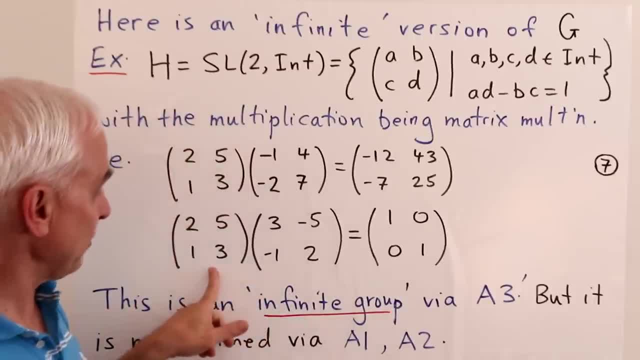 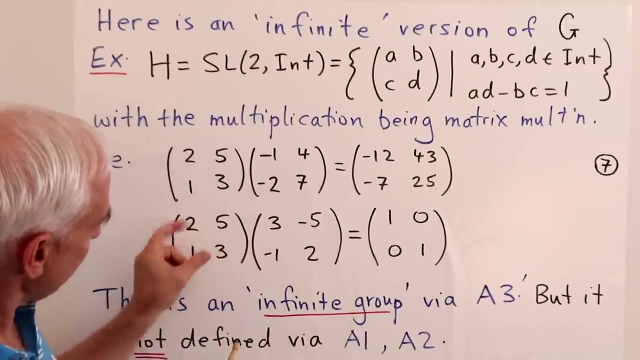 And you can also check that the inverse of one of these matrices is also a matrix of the same type. That's an important observation. And so it's nice to note that the inverse of such a 2 by 2, determinant 1 matrix is obtained by transposing the diagonal elements. So they swap places. 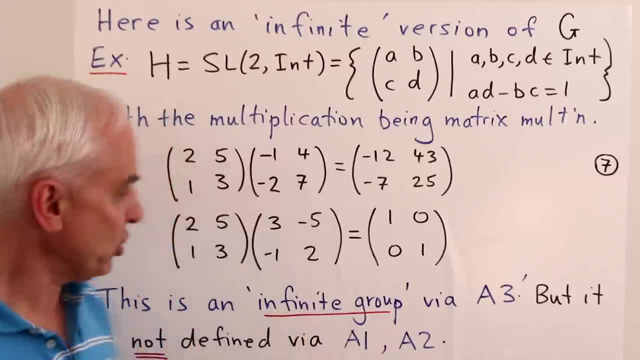 And the off-diagonal elements get multiplied by minus 1. You can check that when you make the multiplication, then, you do get the identity matrix. Okay, so this is a very interesting group. 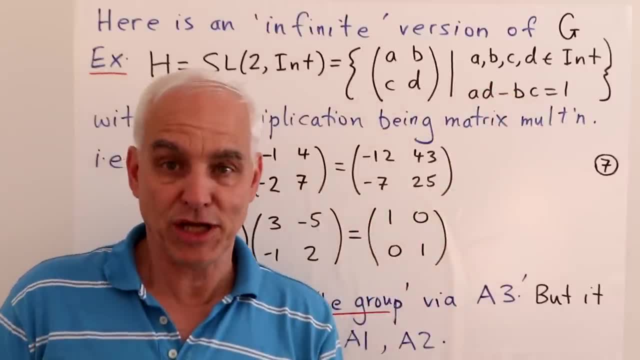 And it's actually a group that's studied very much in number theory and in geometry as well. So it's a very important group. 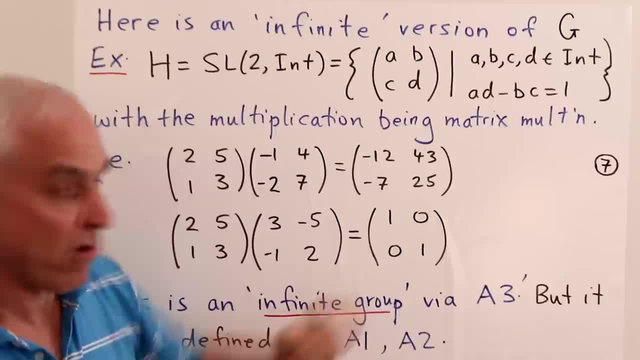 But it's an infinite group via this A3 prime. 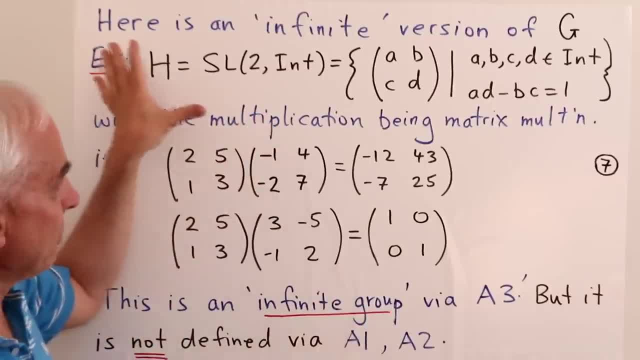 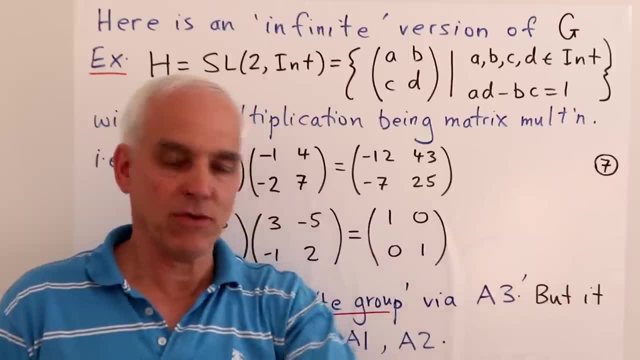 So in modern mathematics, we do not have any problems with making a definition like this. So this would be absolutely routine kind of definition that you would find in mathematical papers throughout the subject. 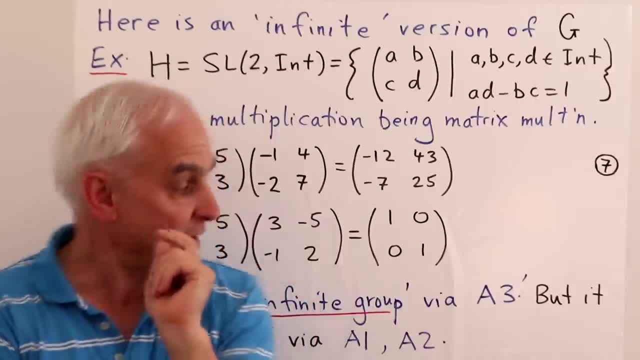 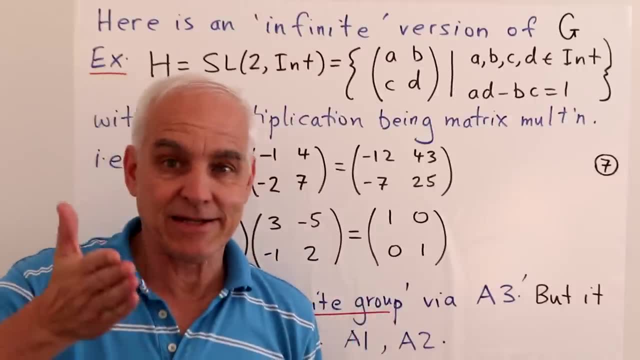 But we are going to look more skeptically at this. Because we recognize that this definition here, this A3 prime, kind of definition, really finesses some key points. 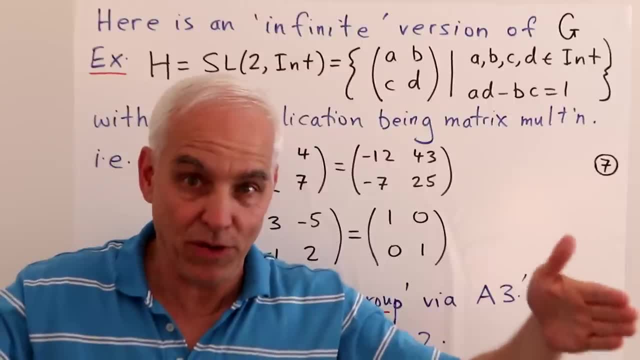 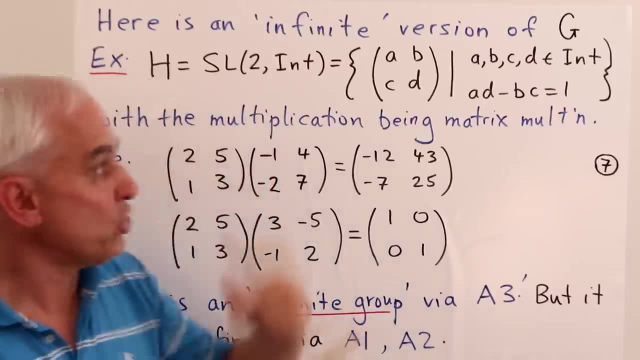 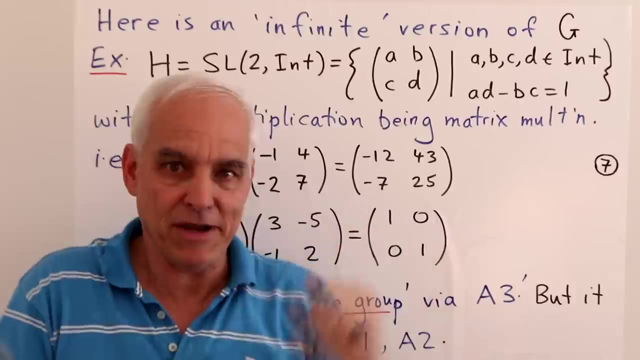 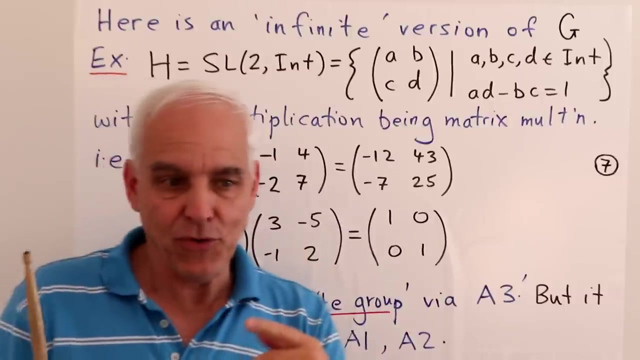 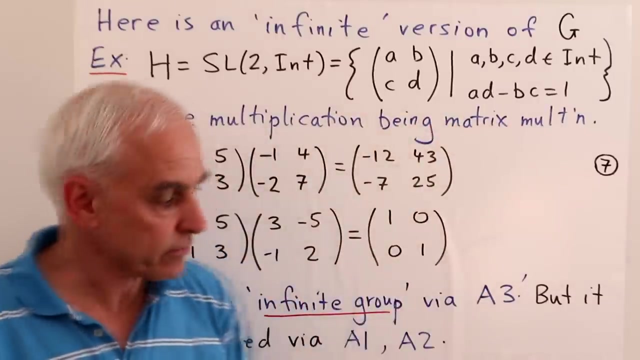 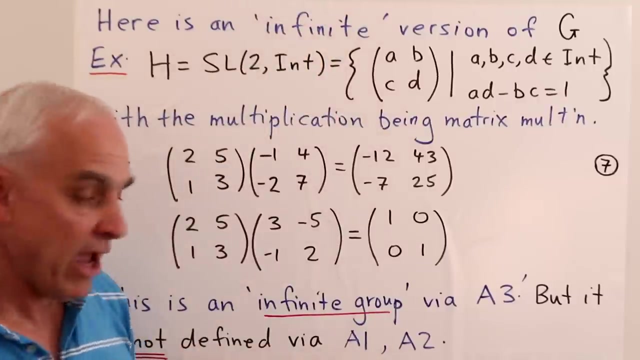 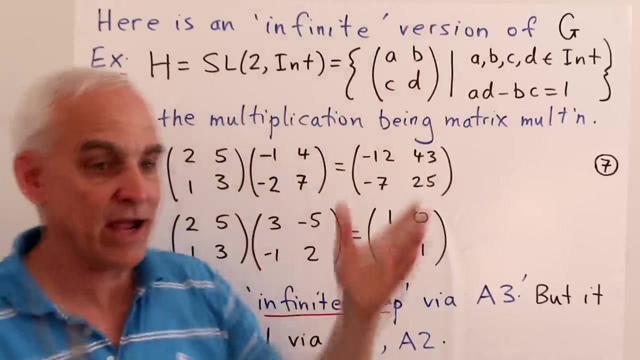 Namely, it doesn't tell us explicitly what all the objects are. And it doesn't tell us explicitly what the multiplication actually is. It's up for us to generate elements. And we're only going to be able to do that, obviously, sort of up to a point. Because there's an unbeautiful number of these determinant 1, 2 by 2 integral matrices. And it's up to us to sort of work out. what the multiplication table is from this sort of basic direction here. So this kind of definition is definitely not in the spirit of A1 and A2, and in fact from the spirit of A1 and A2, if you had that as your orientation, you would not be able to take this and to transform it into something that was meaningful to you. 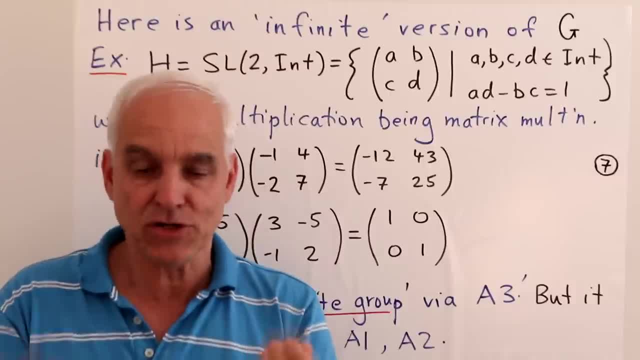 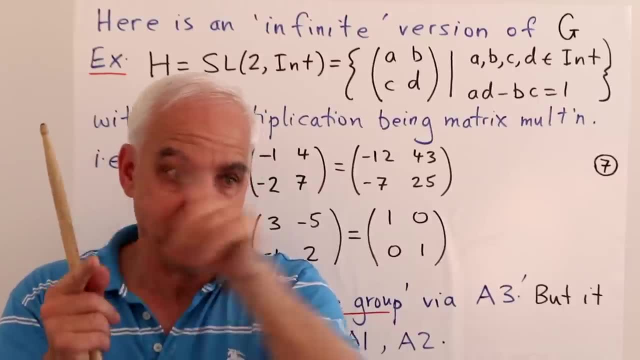 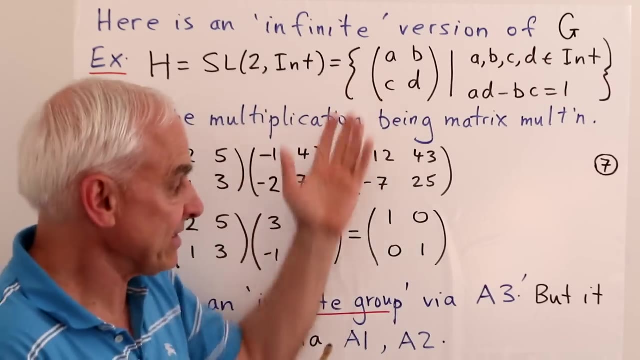 If you're a computer that has been trained to understand that a group is an array, indexed by 1 to k, 1 to k, it's a k by k array with certain properties, you're not going to be able to express this in that language. 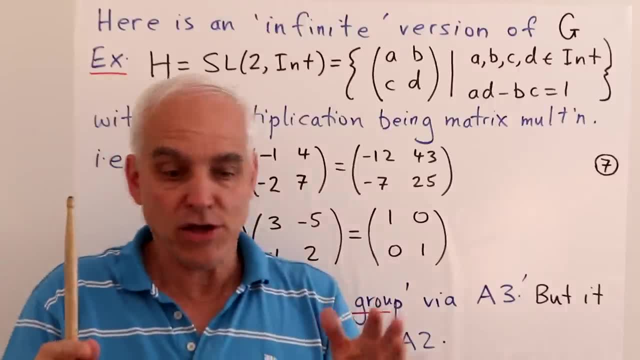 Similarly with the A2 definition, even if you're allowed to not use the numbers 1 through k, but rather some arbitrary kind of set. You're still not able to list all of the elements. 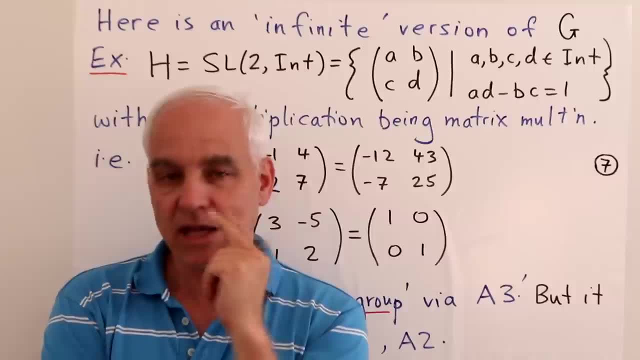 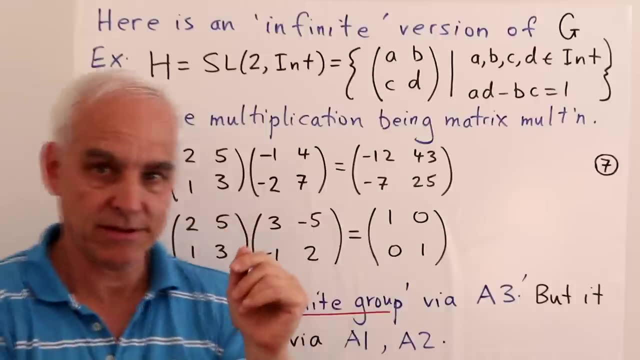 And when we start thinking about things, when we start thinking especially with the point of view of bigger numbers, we start to appreciate that a lot of these matrices inevitably are going to end up involving very big numbers. 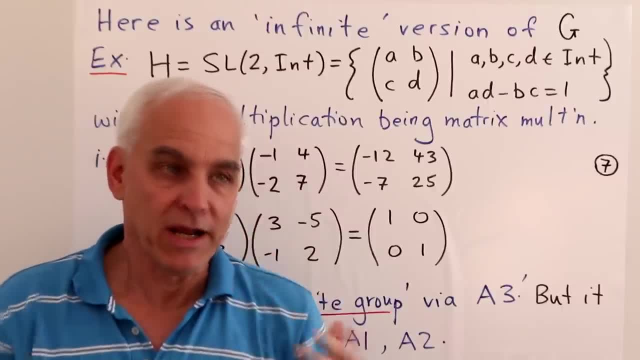 And then we run into the same kinds of problems that we do when we're considering the set of numbers from 1 to z. 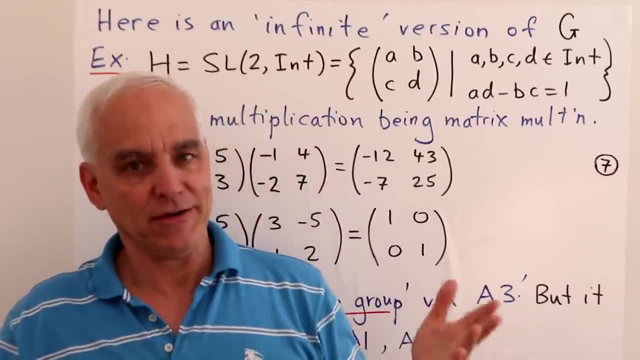 We've talked before about this, right? What does it mean to talk about the set? The set of numbers from 1 to z. 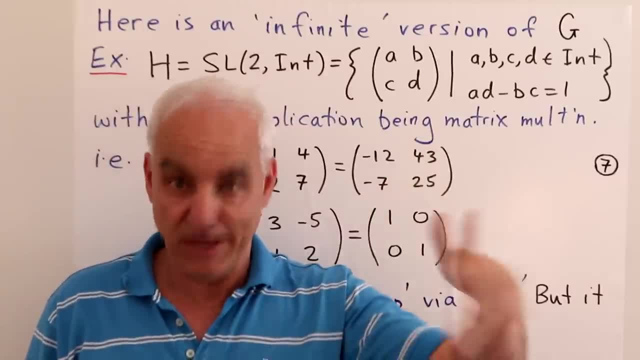 Because we know that most of those numbers are too big to fit into the known universe. They are completely invisible to us. 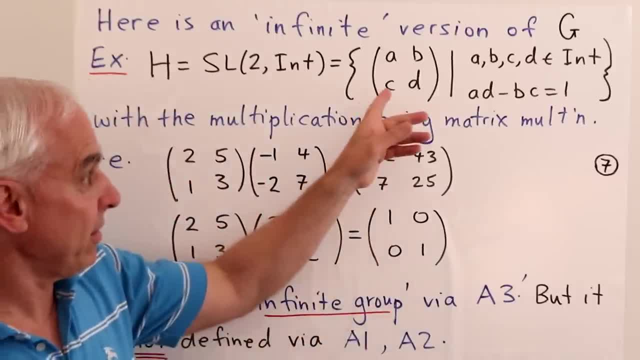 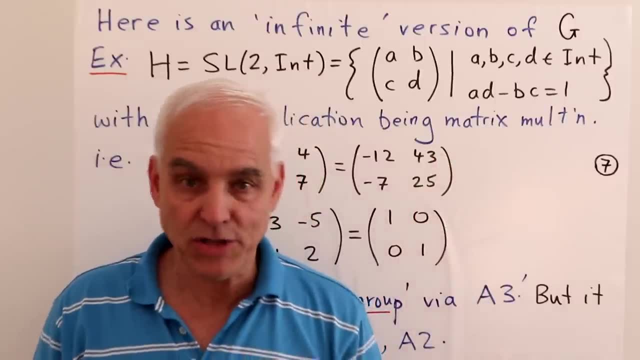 Well, very similarly, that's going to happen with the entries of this group as well. Most of these matrices that we're going to end up considering are going to have entries which are so big that they don't fit into the universe. So exactly the same kind of problems. 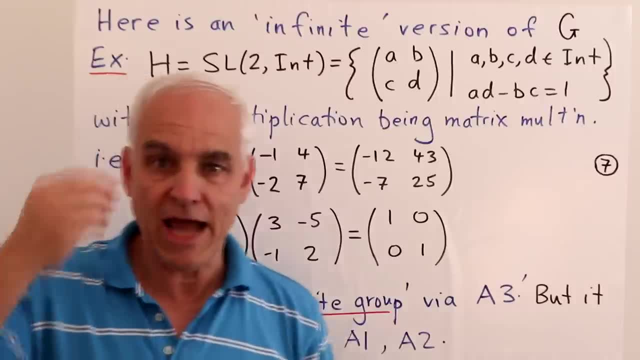 They are going to occur here, that it's no longer clear that we really have control over all such matrices. 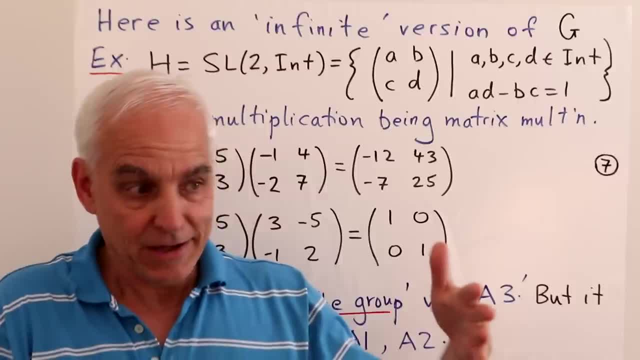 In reality, we only have control up to a certain point, up to the point that we're able to do arithmetic. 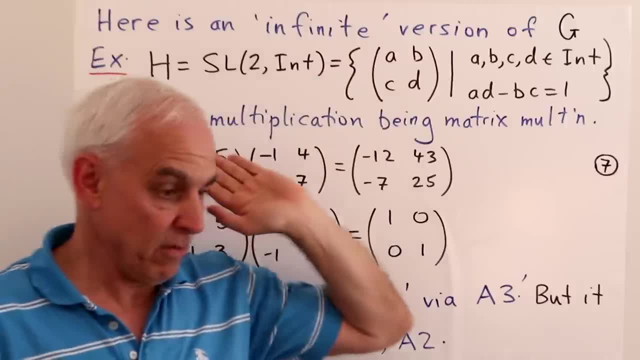 But here we're positing that we are going to consider this whole thing even beyond the limits of our arithmetic. 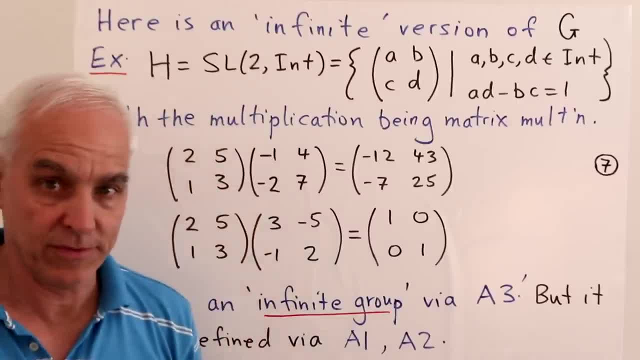 So from a computational point of view, this is fraught with difficulties, but modern mathematics doesn't. 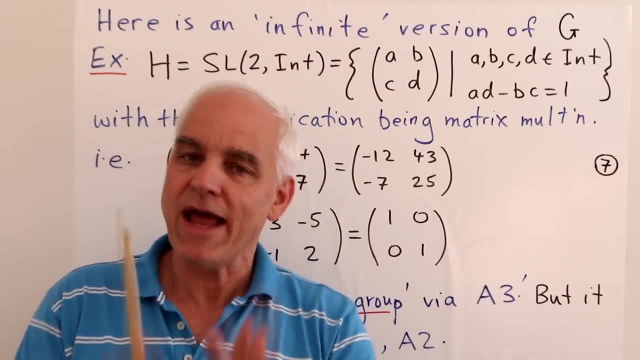 Doesn't recognize that. Doesn't see that because it's quite happy to allow such sort of sloppy definitions. 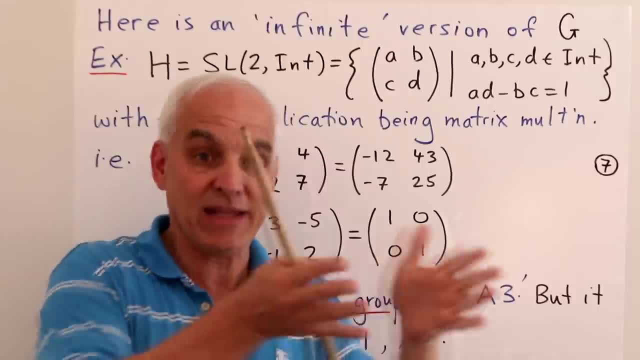 Because for one thing, it makes it easier to make this transition from finite to infinite things. 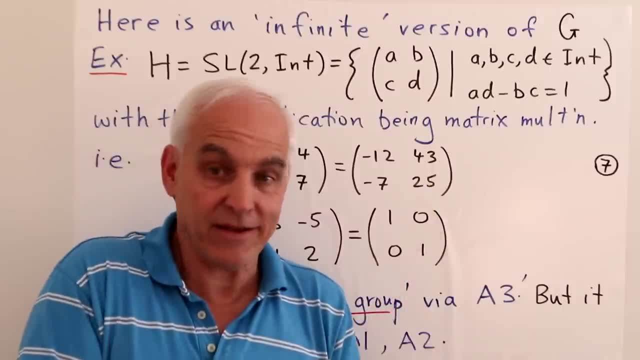 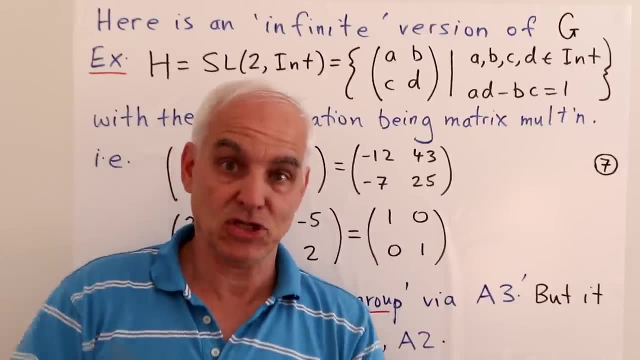 Because if you're not going to be concrete about specifying stuff, then it doesn't really matter if you become a little bit more sloppy by introducing an infinite number of things into the story. Infinite number in quotes. So let me phrase what we've been talking about. 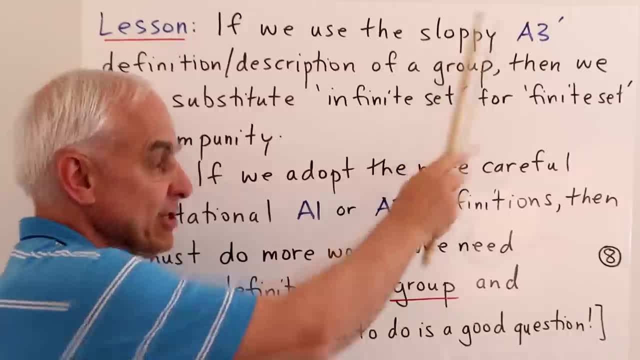 What we've been discussing in the following lesson. That if we use the sloppy A3 prime definition or description of a group and I'm inclined 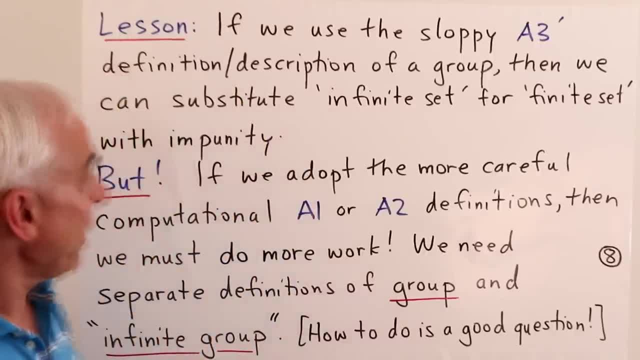 to think of it more as a description rather than a definition, then we can substitute infinite set for finite set with impunity. 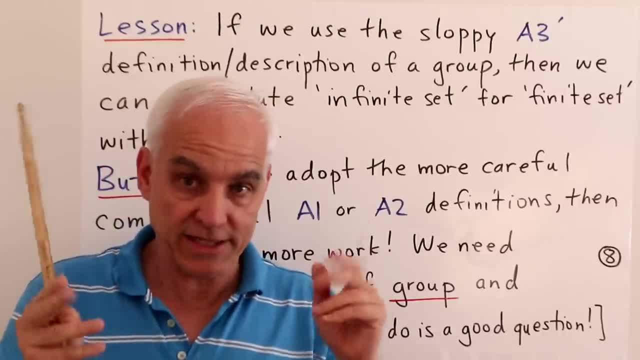 Because part of the whole story is that we are not being careful about what the word set means in the first place. 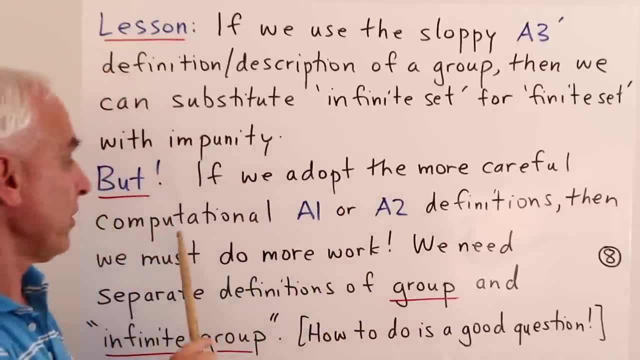 But on the other hand, if we adopt a more careful computational approach. along the lines of the A1 or A2 definitions, 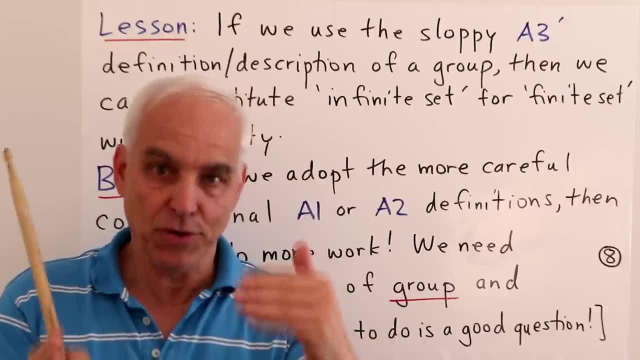 which are geared more towards what a computer can understand, then we must do more work. 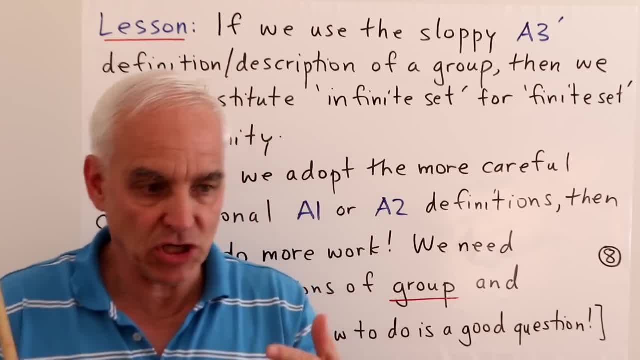 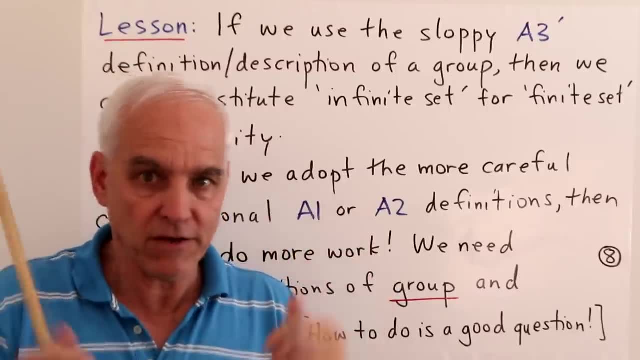 If we want to go from the finite group definition to an infinite group definition, it's not enough just to replace the word group or finite group with the word infinite group. 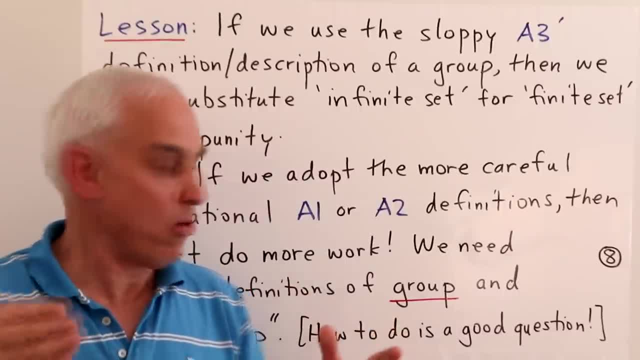 We must actually understand things from a different point of view. So we're going to need separate definitions of group and infinite group. 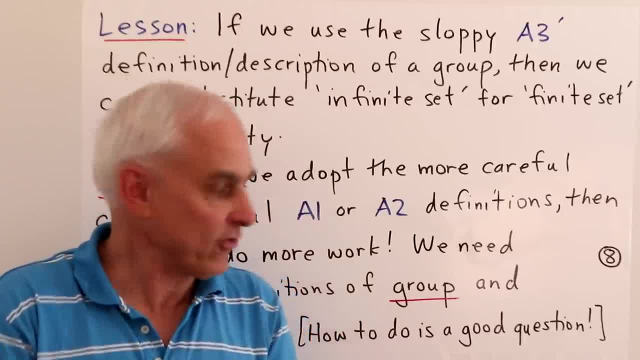 These are not going to be things which are found in the same basket. How to do this is a very good question, and we are going to talk about that. 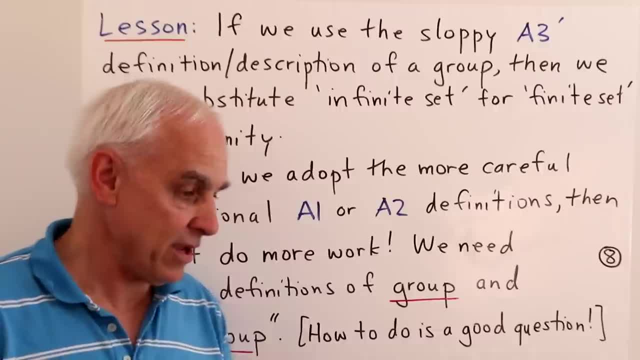 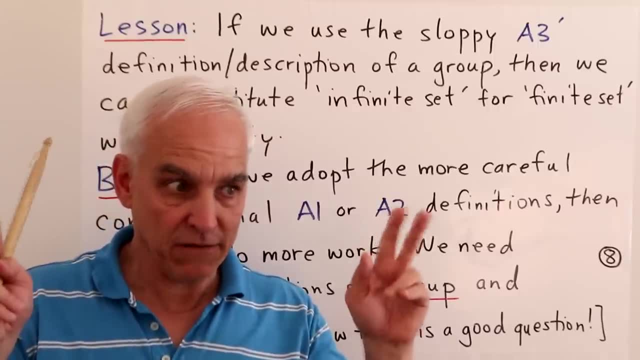 But at this point, I just want to flag that there is a big jump, if you're going to do things properly, between understanding finite, concrete, explicit objects and infinite versions of them.